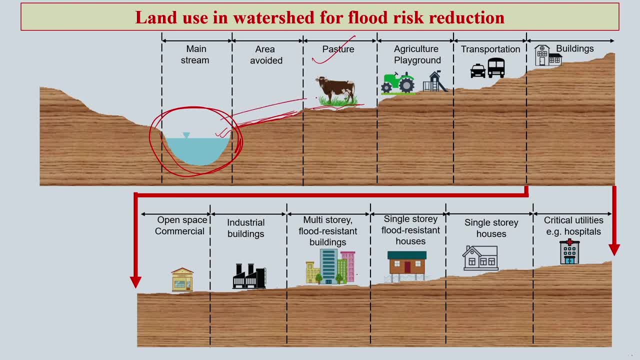 the soil erosion. It can also reduce the speed of, you know, flood water intrusion towards the, you know, land area and also livestock can also be grazed. After pasture, we can have agriculture area and, as well as you know, playgrounds for community. Now, this is the area. 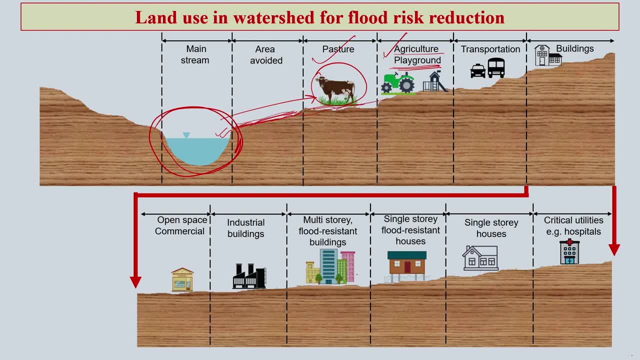 where you also need to assure the supply of water, and at the same time you should be also little bit sure about that frequent intrusion of water from the river or from sea line will not come inside the agriculture land After agriculture land. ideally we should have transportation. 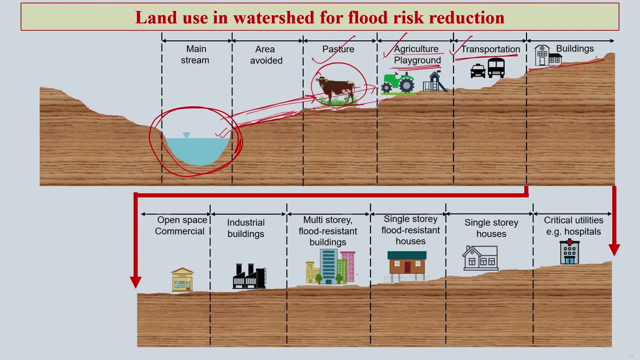 roads and finally your buildings, starts any kind of building, office, school, and you can see that in below picture here. So what are the different kind of buildings and how it should be placed Now, commercial first is commercial group. Commercial type of building should be created in. 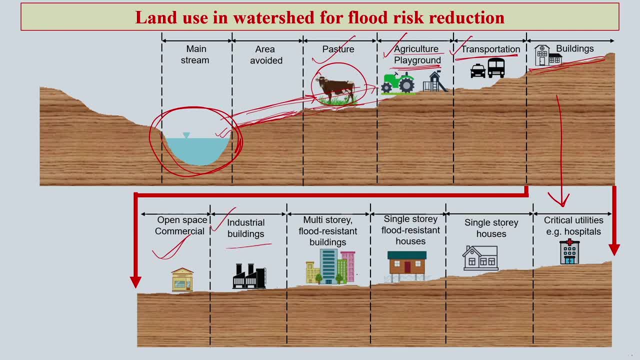 in open space. Then we can have industrial buildings. I am talking about this type of building within this particular land use for building, which should be farthest from the mainstream. After industrial building, we can have multi-story flood resistant building, which could be. 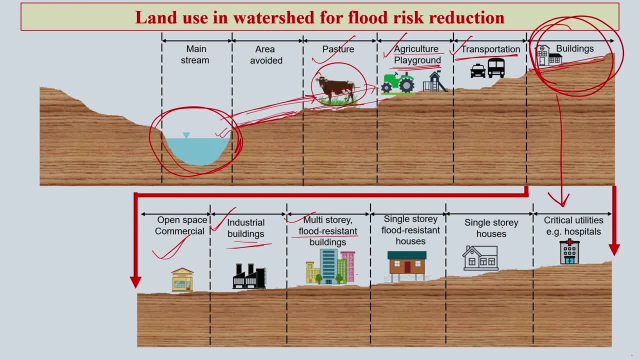 building like flat for people to reside there. It could have office space also there. So, multi-story building, flood resistant building you can have next to the industrial building, Little bit more inside you can have single story for resistant houses. Then you can have single story houses because this is. 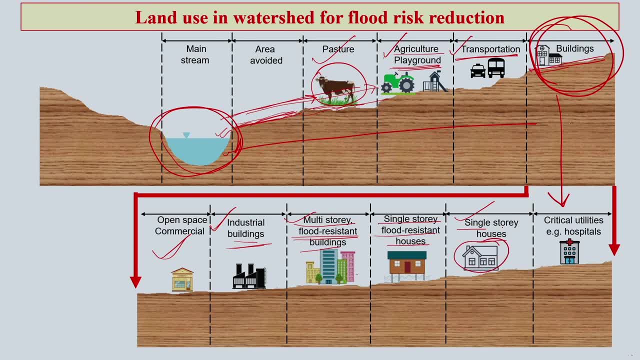 now is bit far from the mainstream. So the chances of flood water intrusion is relatively less. Finally, you have critical utilities like hospital, because we need to ensure that such critical facilities must be far away from the chances of any kind of flood water intrusion. So this is how. 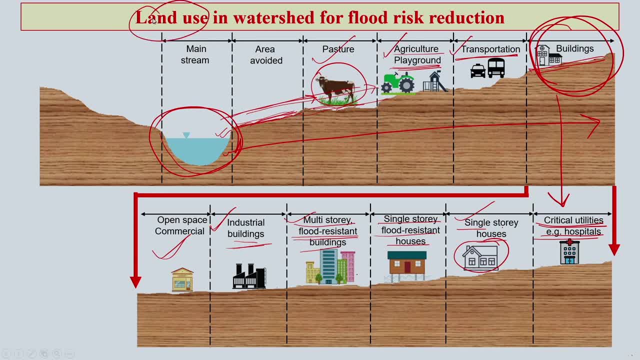 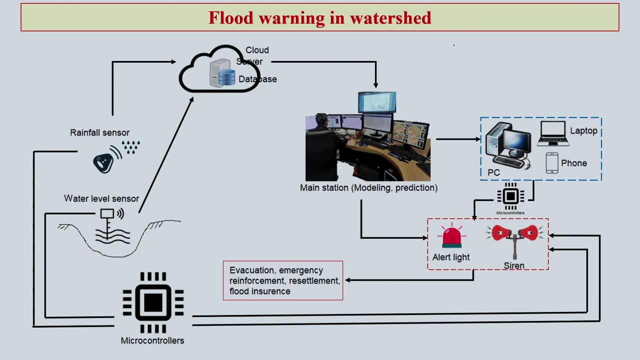 you choose the land use and, accordingly, you place them to reduce any kind of risk that may occur from flood. Now, early warning system, EWS. Early warning system is a very, very important aspect for anything, whether it is flood, drought. 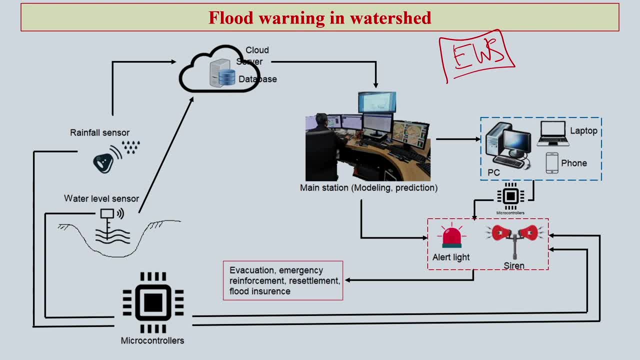 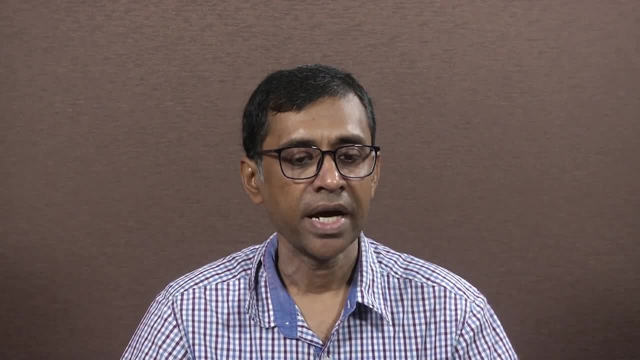 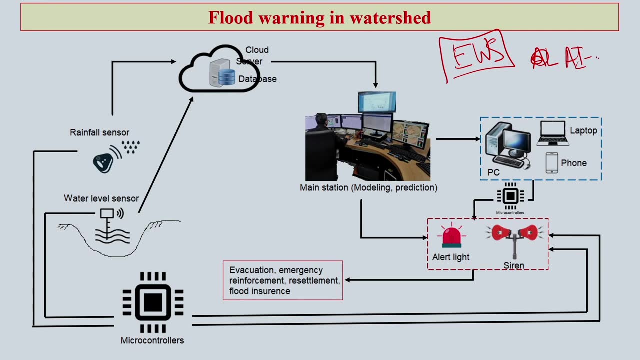 cyclone, anything, any kind of natural calamity that you can think of. Early warning system is very critical, you know, for saving life and other resources. Now uses of advanced technologies, artificial intelligence, machine languages- these are the advanced technologies. EWS is one of the most advanced technologies in the world. EWS is one of the 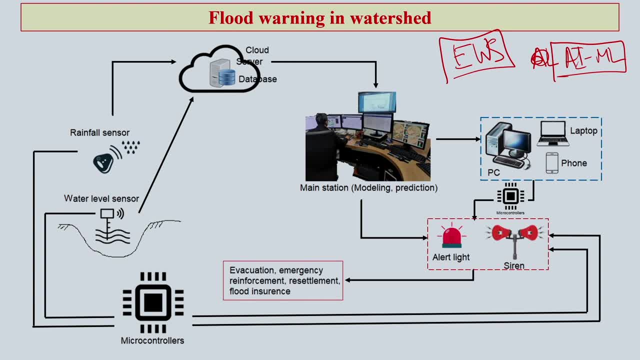 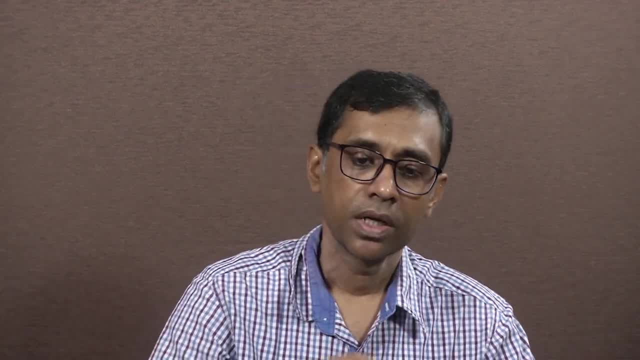 most Exceptional technologies in the world. EWS has been used in a wide variety of ICT: clutch, cloud software, cloud services. It has been used for a large number of all these types of technologies. Now you can have these kinds of data due to the many features of EWS. 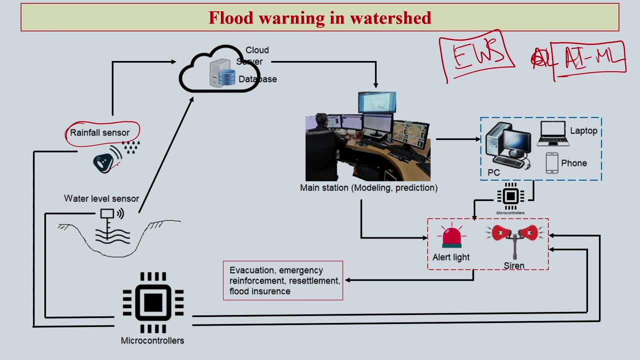 You can have all the information. you can have all the data. you can have data that you need in a single place in the world, and then you can have all the information about EWS. You can have all the data. you can have all the information about EWS, which these days are. being utilized for developing efficient early warning systems. Now for flood. how actually it works. Now. you have some sensors, which starts from any basic steps. You have some sensor- rail phone sensor- which can actually detect and can send the signal to the server which you have in cloud, and also the database are created. Apart from rail phones, you can have the cloud and also the database are created. 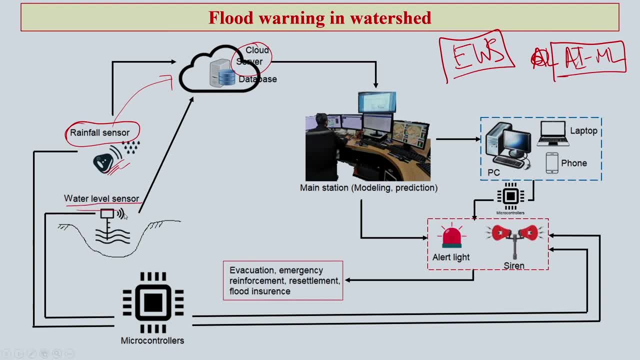 phone sensor you can have also. water level sensor means this is the sensor. So if your water level rises beyond a certain limit, it will automatically send a signal into the server and that data will be stored there. From the server the information will go to: 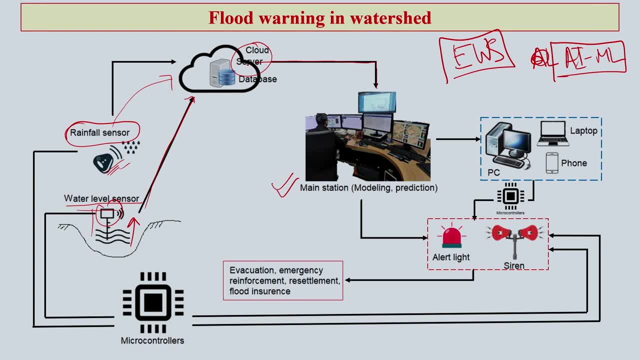 the main station where a person or a team of person with continuously monitoring that and then they will utilize those sensor through some modeling and then they will come up with early warning or prediction of an event. Now this main station has actually all the kind of you know machines that you need and these machines actually, you know, largely regulated. 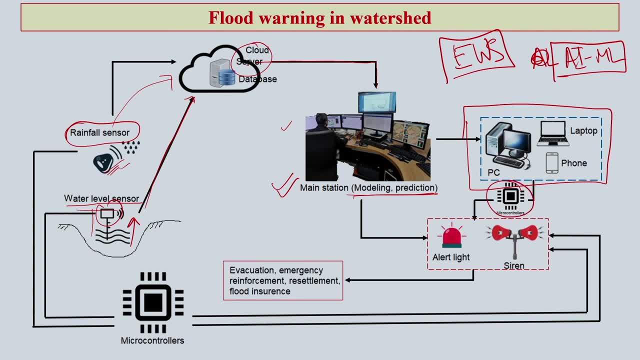 by several kind of microcontrollers and these microcontrollers will provide some kind of you know warning, either through you know light system or through sound system. Now the information which actually generated from the field through sensor, Now this information straight away go to the server, come to the main station, processed here the information. 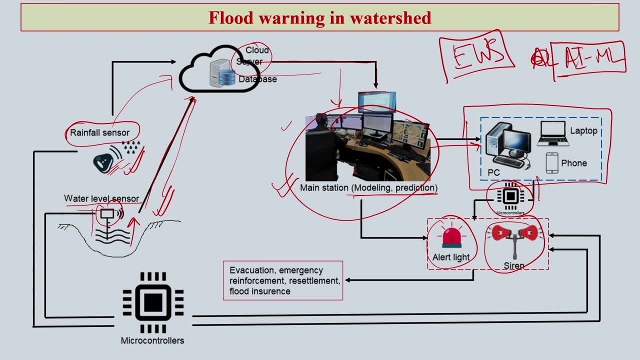 goes to the systems. from the systems, the you know message goes to some microcontrollers and then they translate it into either system. So this information goes to the people, to various stakeholders, state disaster management authorities, people who are involved with evacuation, So they get alerted and then accordingly, 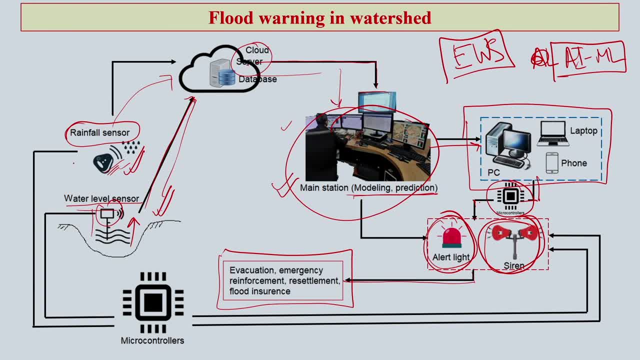 the actions is being taken Now here is another way: that from the sensor, as I said, the information can directly go to the server, but the other part, from the, both the sensors, say rainfall sensor or water level sensor, it can also go through sets of 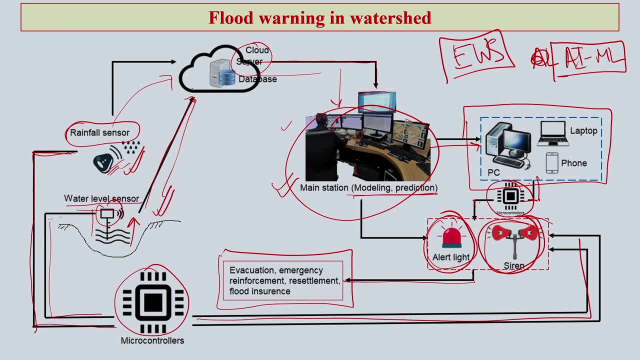 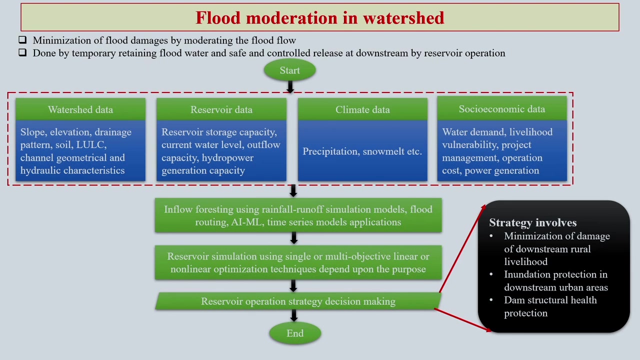 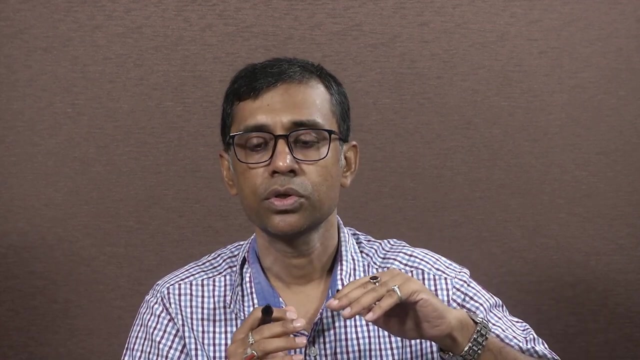 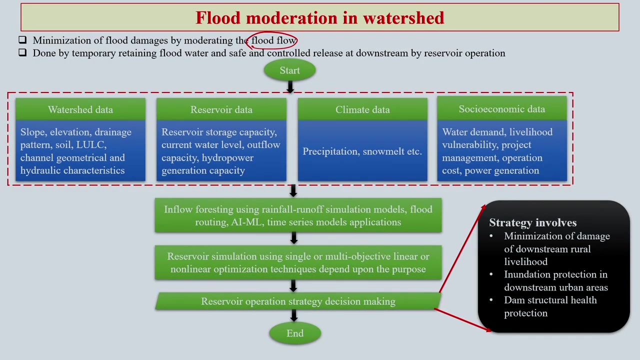 microcontrollers straight away to the warning system. So this warning would be, you know, kind of what you call live early warning or live warning system, or you can say real time, real time warning, And then finally the process of moderation will start. So in watershed level you will. 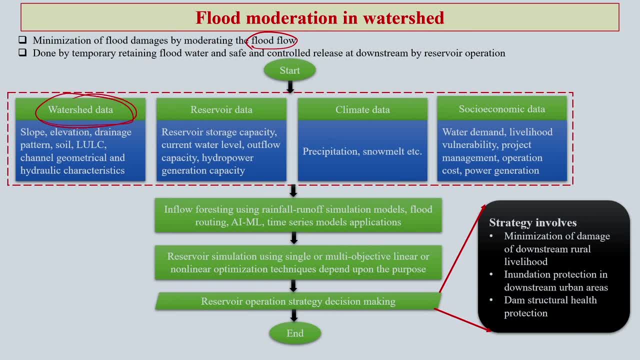 have some data, as I just mentioned in the previous slide. it could have and in the cloud, or it could have in the server or in different manner. Now, watershed has certain information about slope, elevation, drainage, land use, hydraulic characteristics, etcetera. Then you have reservoir. 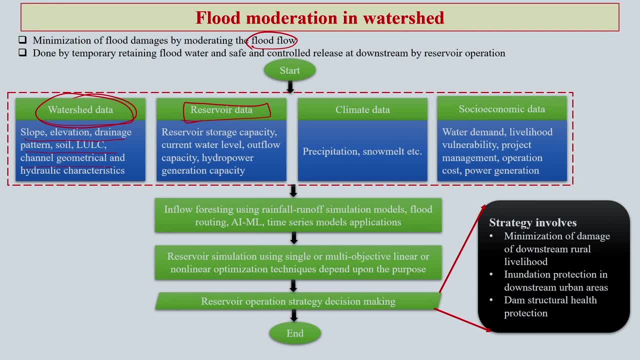 in that area. you have also information about the reservoir storage capacity, current water level, outflow capacity, hydropower generation capacity. You also have with you the climate data, which talks about precipitation, wind, etc. Then you have socio-economic data, where actually you. 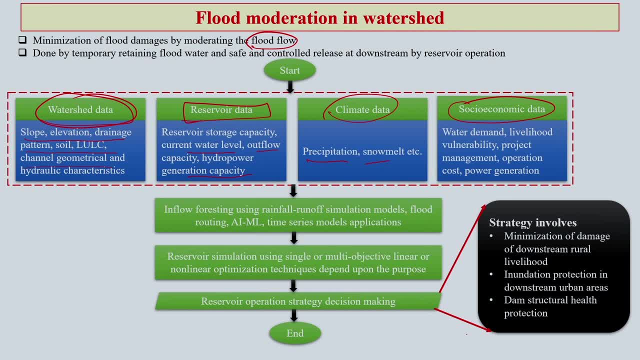 have the information about the water demand, the livelihood vulnerability, the project management system, operating cost, power generation. all these information you have under socio-economic data. Now, once you have these all data or information with you, then you actually using this rainfall. 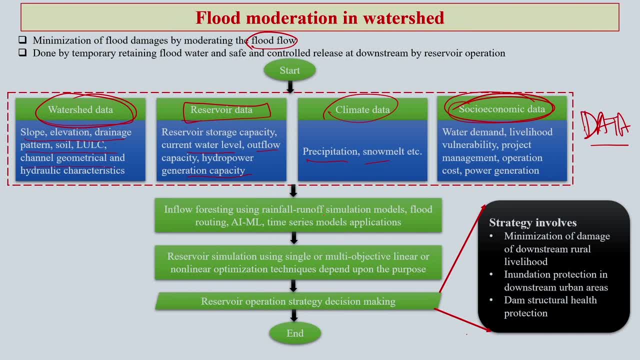 and runoff data. you go for simulation models: flood routing, you use AIML and different kind of time series models applications to come up with some kind of anticipatory solutions Now, reservoir simulation using single or multi-objective landscape. So these are all. linear or non-linear optimization techniques also are there, but they depend on your. 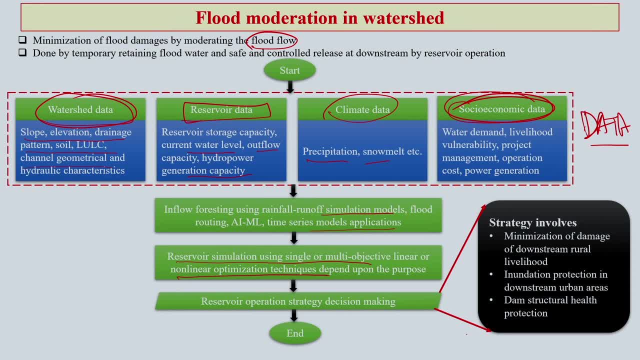 purpose. There are various options, So which one to go for actually will be decided: the purpose for which you are going to use that. Now, once you analyze all these data that you have and through this you run some model, come out with some kind of decision support system, then you get. 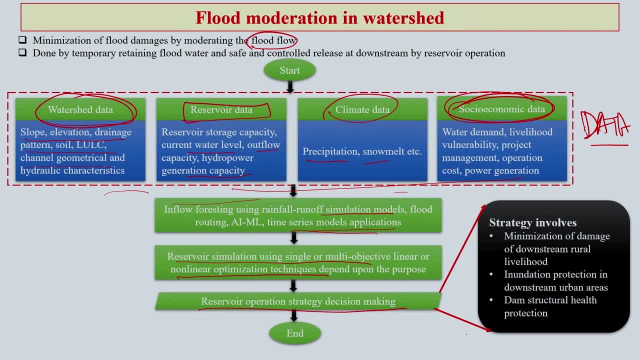 the reservoir operation strategy. decision in the process, on the basis of this database which you have with you and through certain- you know- advance analysis of those data. finally, you come up with a strategy. One can call it as decision support system, DSS. Now what? 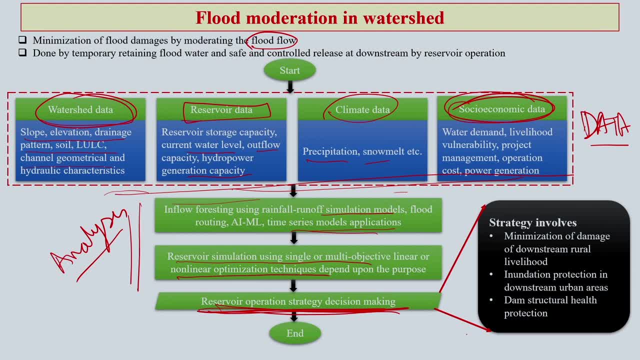 actually at this stage- you know the strategy or decision making stage- What actually are involved in that particular processes process minimization of damage of downstream for rural livelihood, because from upstream when you see the water level goes beyond safety limit, certainly you have to decide to allow some water. 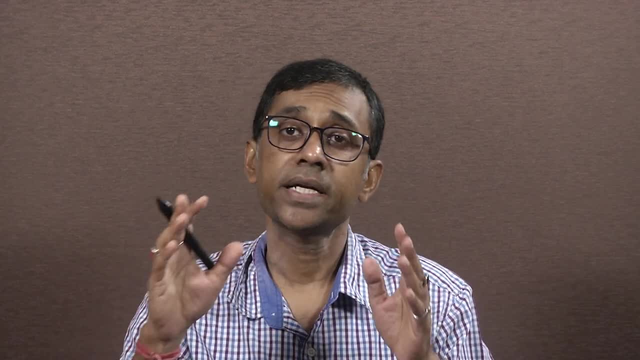 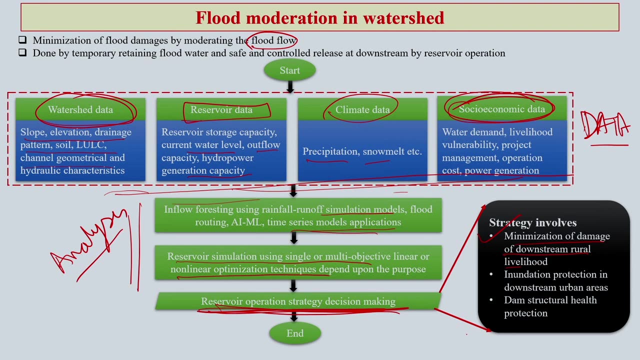 to go to the downstream. but that amount of water which you are going to, you know allow to pass towards the downstream, also depend on that the livelihood, the agricultural areas and other aspect which are actually located there in the downstream. so you have to consider the impact of releasing the water towards downstream beforehand. so minimization of damage of downstream. 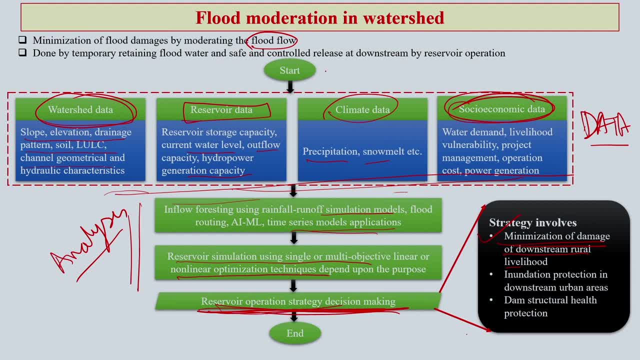 in the rural livelihood can also be decided through this kind of exercise which i just expressed. then inundation protection in downstream and urban areas. often it happens that it is not because of the rainfall that the downstream area is getting inundated or flooded, but it gets because the water has been released from you know some dam or 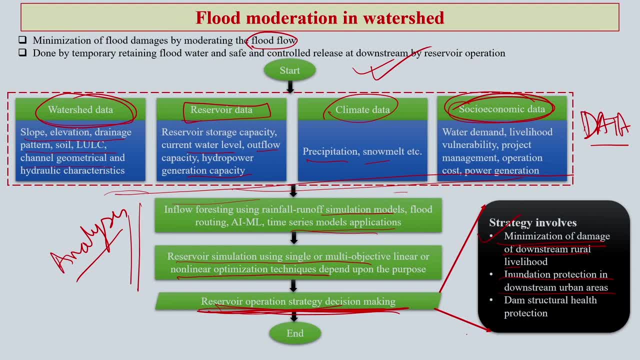 or some place where you have a reservoir, so that decision has to be, you know, taken considering upstream as well as downstream condition. dam structural health protection is also another aspect which actually taken care of in this process when you make the decision. so, coming back to this, that the entire flood moderation system, which is very, very important, 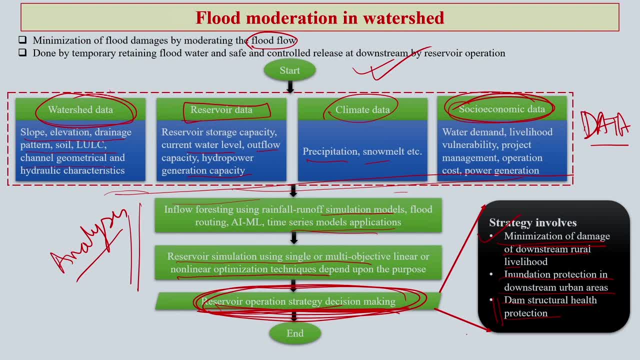 for any watershed. we start doing it with the help of the data that we already have, and these datas will actually go into different kind of modeling systems and then they will analyze that. that information will go ultimately through some optimization exercises to be sure that, yes, what you are going to do is you are going to measure around the stream and then you can say that this is. 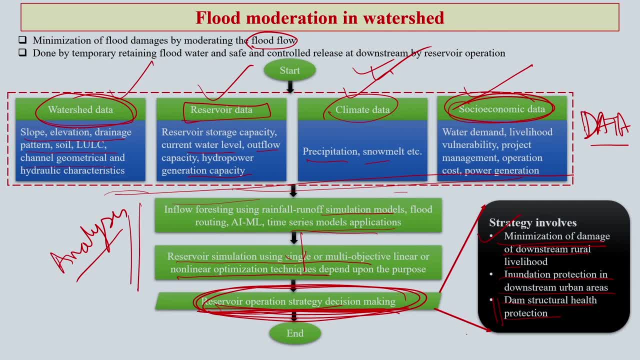 you know the river, so you will measure from what. what you are going to do and you can also do going to give the decision is almost error free, because any decision taken there could affect either upstream or downstream people infrastructure resources. So these are the aspect that we should keep in mind. 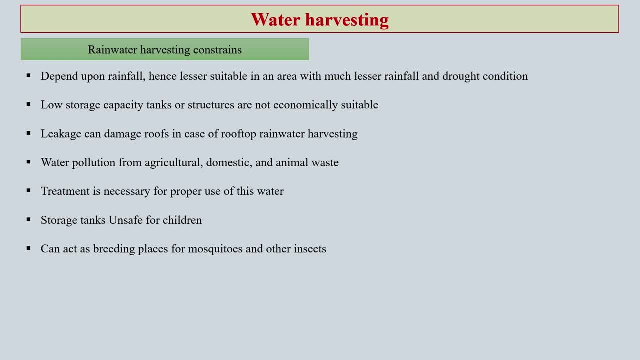 I earlier talked about water harvesting issues. I also discussed about roof water harvesting and why it is important even in area where good amount of rainfall takes place. Those things I have discussed Now few point I just thought of. you know, sharing with you is that water harvesting is good. 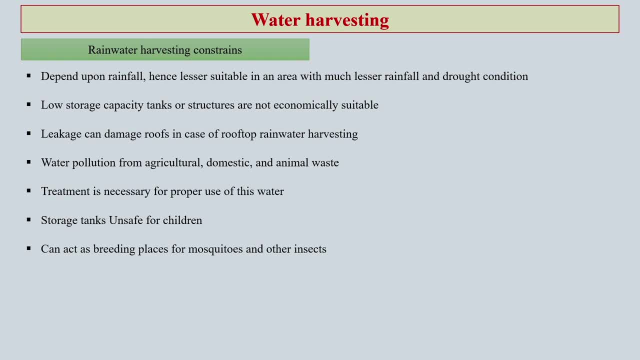 we know that. But there are certain constraints that the practitioners or administrators or community, when they go on the field to do it, they may face this constraint and they are like rainfall, So it largely depends on the amount and frequency of the rainfall. So water harvesting. 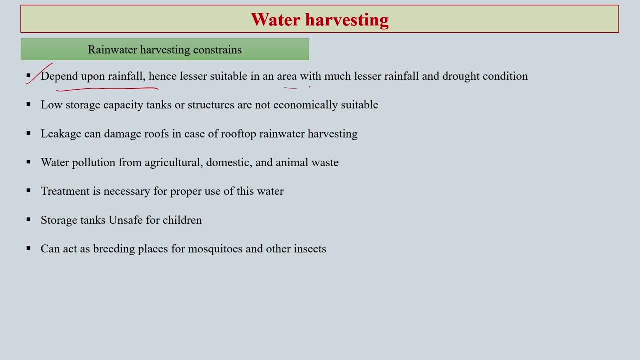 Generally is not much suitable in an area with much lesser rainfall or drought condition. we know that. Second, low storage capacity tanks or structures. they are not economically suitable for water harvesting. Third: leakage issue. If you have leakage issue, then your entire effort, investment energy for having water. 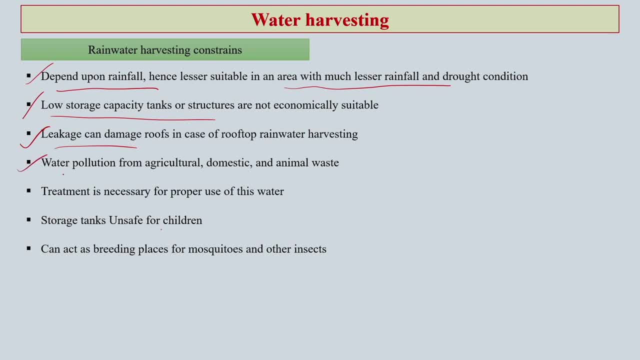 harvesting could be a failure: Water pollution, Water pollution- Another aspect: you have, suppose, successfully done the water harvesting, stored it, But the water that you have stored if it is already contaminated then it is of no use. So it is important to see the water pollution level and surrounding agricultural domestic. 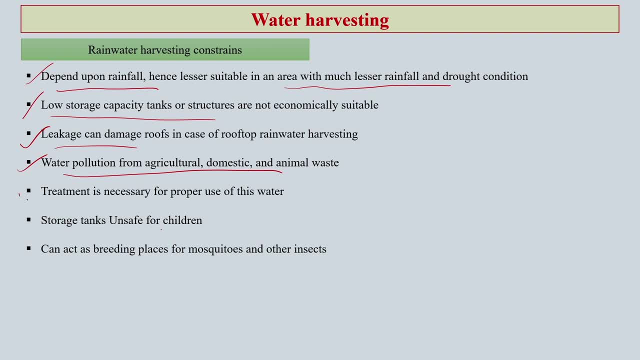 and other waste nearby to that area. Treatments is necessary for proper use of the water that you have harvested. Sometimes storage tank After a�taa is placed in that storage tank it is pottery or old junk which can be fully pressed, much released itself. 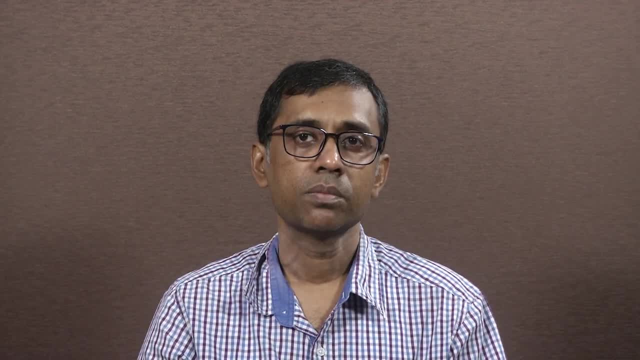 Sometimes it is pig mummy because of the vessel. it can still be seen Inちack and dica and many other. such A lot of illegal material If we come to the grains of the grain. if we come to the grain of the grain, it can. 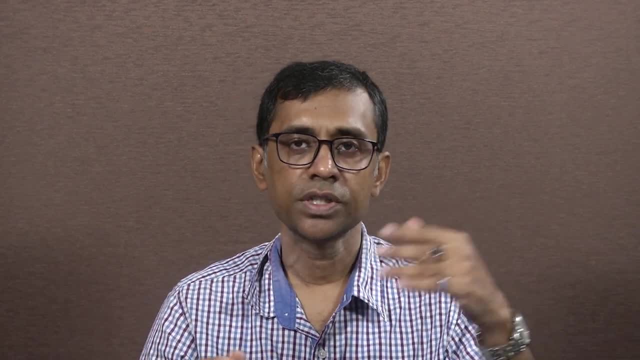 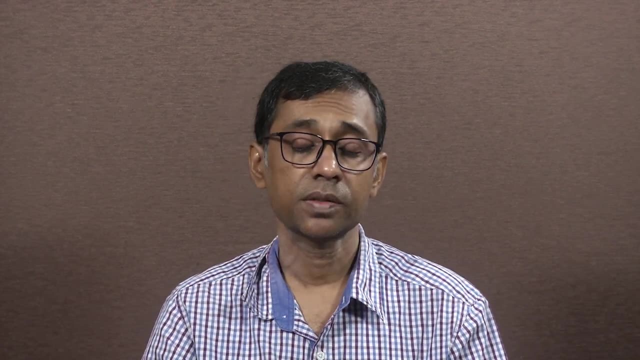 give this the source, becomescuz this all this. You have this organic mixture, It can bring. There are also these for benefits: to produce the, But do not put it in the landfill tank. It voraciously like actualということ of the soil. 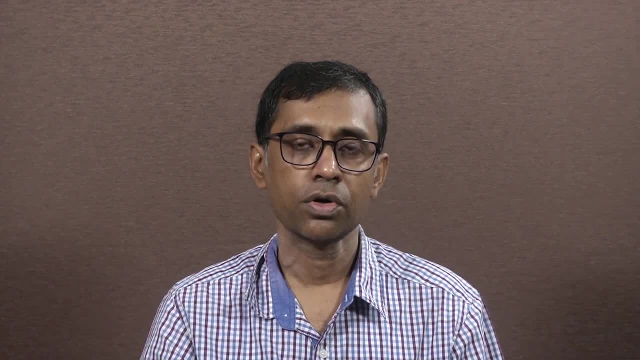 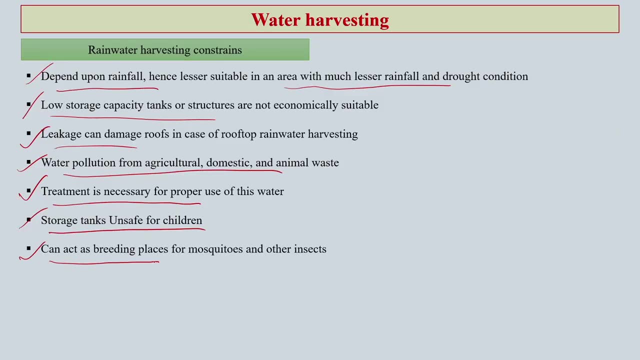 We do not do. the manual process是 German word often mentioned. again one very practical issue or constraint, then often you might face it in case of water harvesting. This can also act as a breeding places for mosquitoes and other insects These days when you have, you know, various kind of like dengue, etc. So clear water is also we. 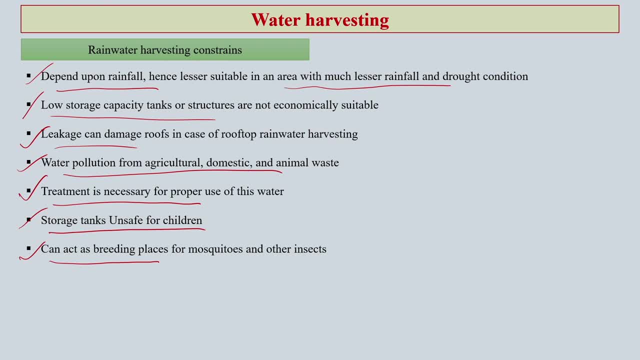 know that is a very suitable breeding place for dengue mosquitoes. So these are few very practical constraints or challenges that we have in our hand that we need to take care of while we go for water harvesting. Now, in case of water harvesting, you will find that at the 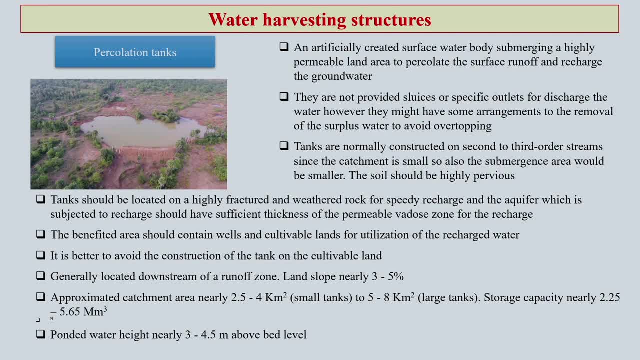 rural level or at the village community level, one of the most common water harvesting structure that you can see is percolation tanks, or in some cases people call percolation port. Now, this is basically artificially, you know, created surface water body, which is highly 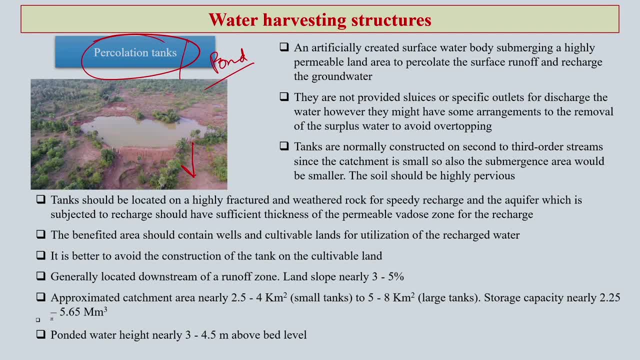 permeable and this should actually allow the water to percolate down below so that it can recharge the groundwater. That is the main purpose of percolation pond. Now, this percolation pond, they are not provided with sluices or specific kind of outlays for discharge of the water. 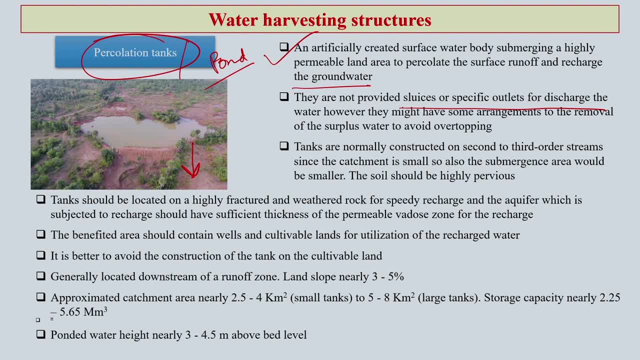 However, this percolation pond is not provided with sluices or specific kind of outlays for discharge of the water. If the water is not provided with sluices or specific kind of outlays for discharge of the water- You know percolation tanks some time could have some kind of arrangements. 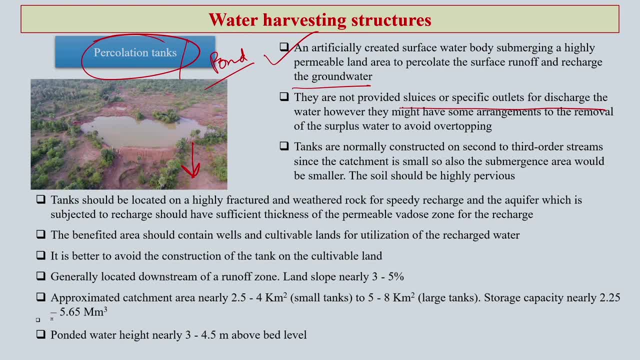 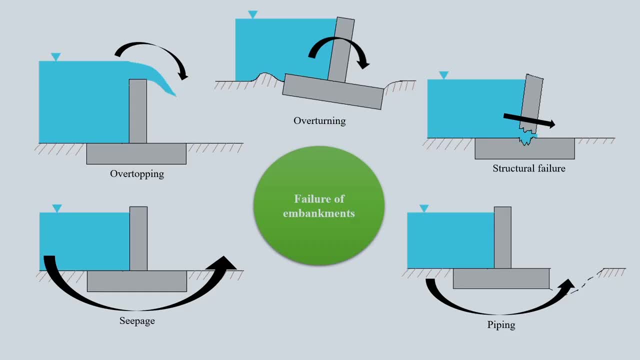 for the removal of the excess- you know surplus- water to avoid, just, you know, overtoping. You remember that that we have discussed about, you know toppling down of system in case of kind of flood situation. So this is what actually as, talking about that overtopping. 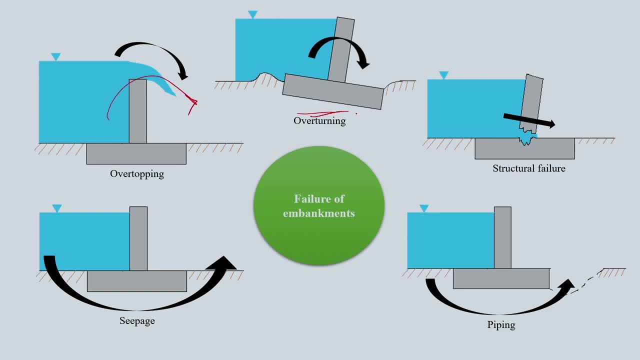 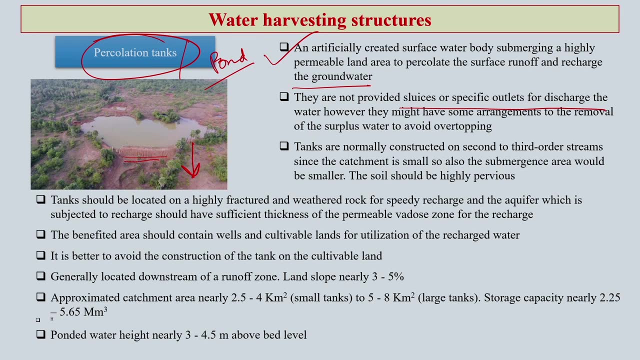 can also takes place. in over turning can also takes place. So this we have to also keep in in mind. now, tanks or ponds- percolation tanks or percolation ponds- normally constructed on second or third water streams. why? because the catchment is generally small. okay, so also the 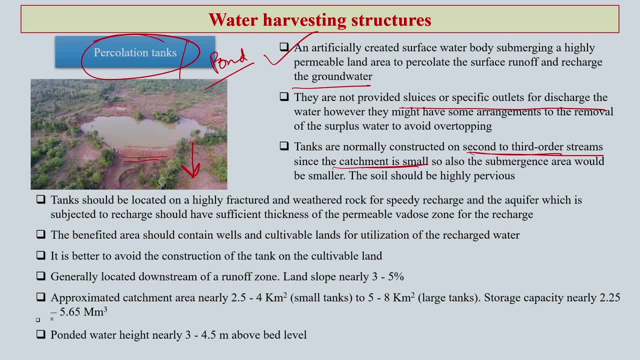 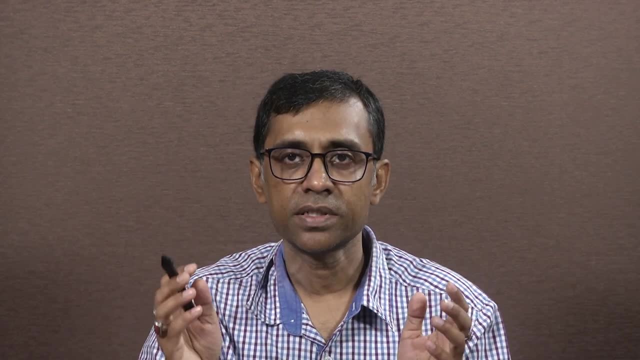 submergence area would be smaller, relatively smaller. the soil needs to be highly percolating in nature because whatever water which is stored in the percolation pond has to go down, has to percolate so that it can basically recharge the groundwater, because that's the major purpose of 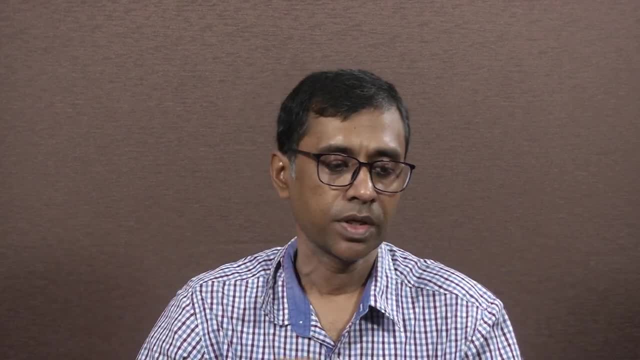 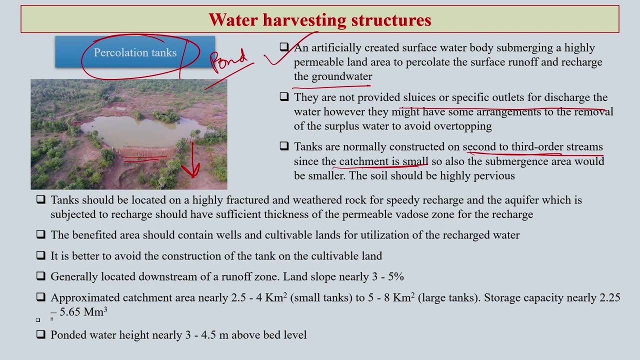 having the percolation pond for water. harvesting tanks of these ponds should be located on a highly fractured and weather rock, again for speedy recharge of the aquifer, which is mostly, you know, a get recharged through this water storage structure. where we see this is from the bottom one, where 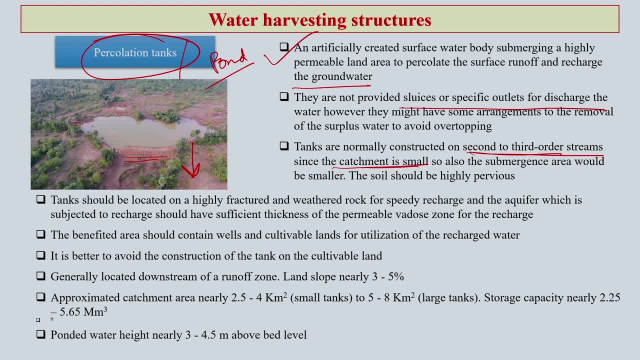 we see these rock once the water has been put in the water purge. so these sample is to be put on this percolating water. So the benefited area, the surrounding area of this percolation pond, should contain wells and cultivable lands for utilization of this recharge water. So 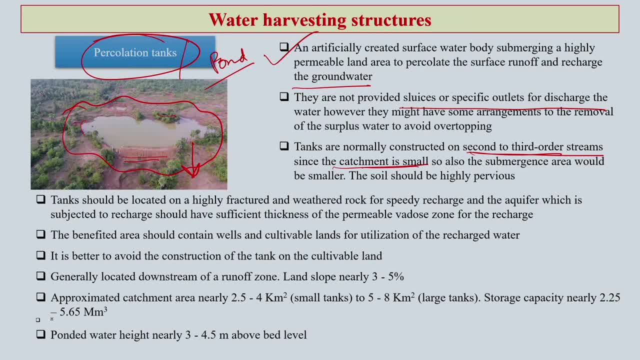 if you have a percolation pond here, ideally you should have kind of a well recharge well here in these areas, And of course this percolation pond should be surrounded by agricultural land because that these areas groundwater is supposed to be already recharged by the 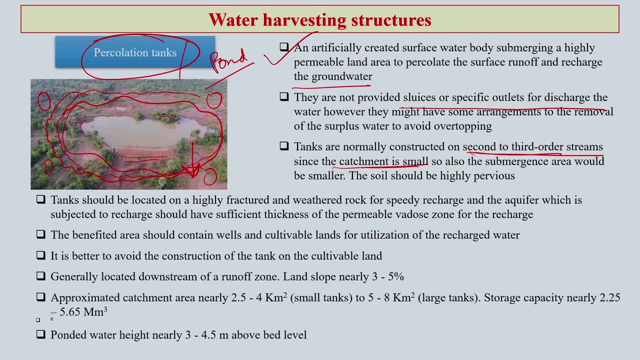 presence of this percolation pond. So the pond water height in general are somewhere on between 3 to 4.5 meter above the bed level. That is an ideal kind of height for such kind of percolation pond. So this is a very simple water harvesting structures but has a 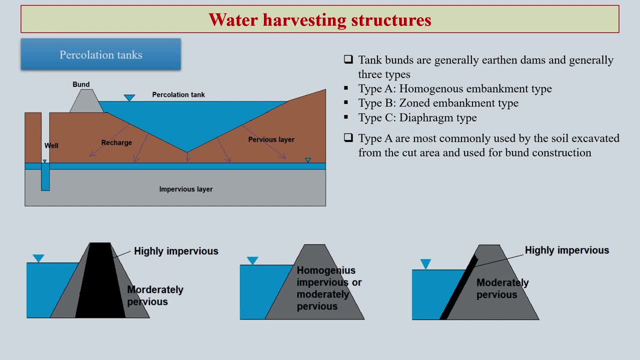 very good effect on recharging groundwater. So how actually it works. percolation tanks. So as you see that this is the picture, it can explain you about the technicalities of percolation tank. So this is the water body. 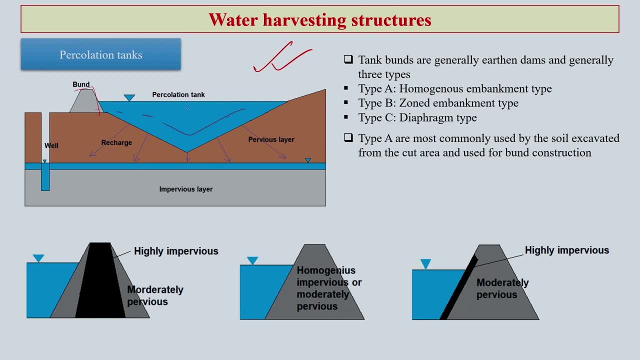 the tank you have. You can have a small bund here in case this water level rises, and should not go there. But even if at a some time, because of excess rainfall, if the water level rises, if the water cross this bund, it can come inside this well and again it can recharge. 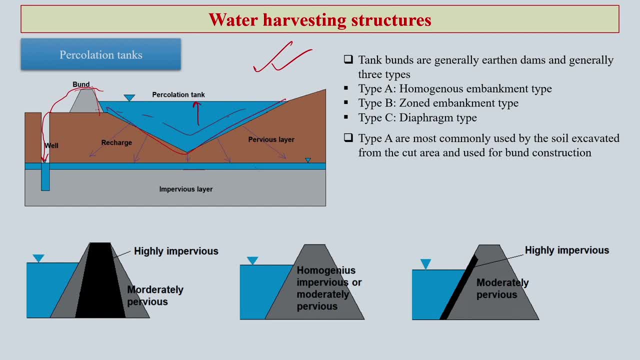 the groundwater. Obviously, this percolation tank, which is already you have created, they will directly recharge your groundwater, as you see these arrows. So they will already going to recharge and, in case of excess water, as I said, they can if they pass the bund. 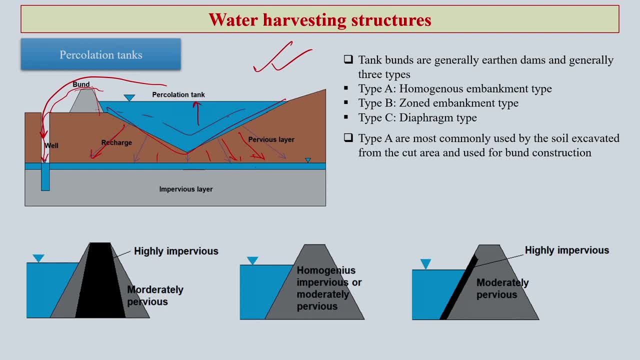 they will go inside the well and again they will recharge the groundwater. Again, as I said, that these areas largely should be pervious layer means water should be allowed to percolate so that it can recharge your this groundwater. So in case of tanks, bunds are generally made of earthen dams are generally three types. 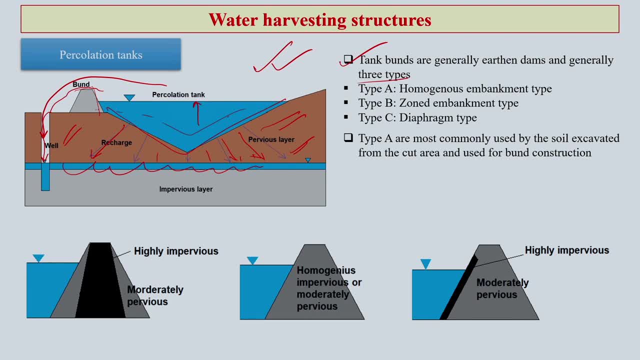 which actually we see in conditions like India and Indian subcontinent. Type A, which is homogeneous embankment type- We have discussed about embankment earlier- Type B- zoned embankment type. And the third type, Type C, is diaphragm type. 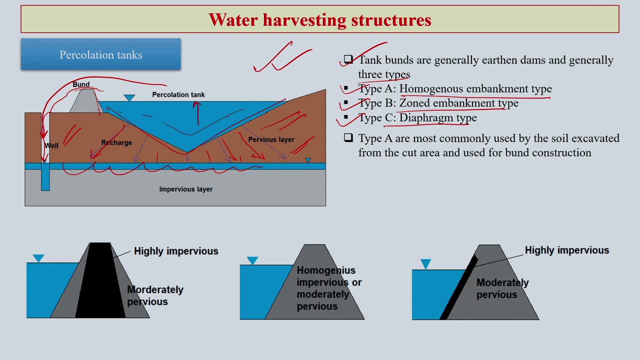 So these are the three types of earthen dams that we normally see in case of percolation tanks, like structure for water harvesting. Among these three, you will find that type A are the most commonly used earthen dams, then dam which is normally created by excavating this particular while you actually 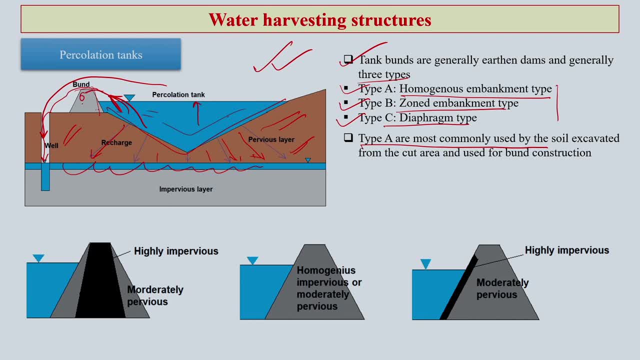 creating this percolation pond, this soil actually you deposit here and you create a earthen kind of dam or bund. So even the soil which is comes out of these excavations are used for making the earthen, you know, bund or dam. 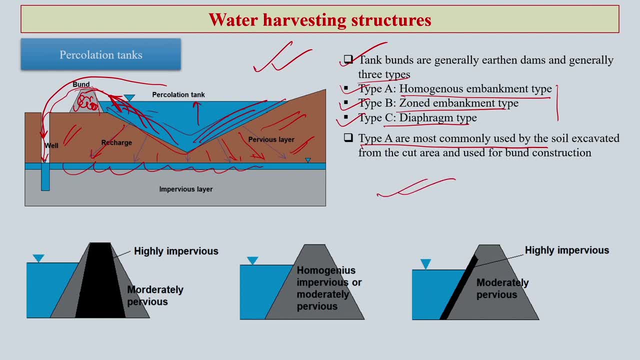 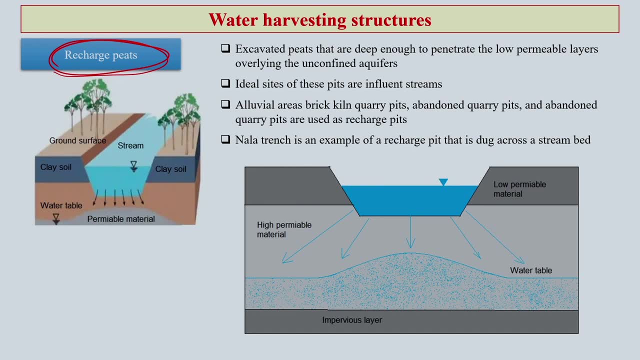 So this is a in brief, is the percolation tank. you know inside detail. the second type of, you know, water harvesting structure at the community level comes recharge pits. Now, recharge pits are made through excavations which are deep enough to penetrate even the low permeable layers overlying the unconfined aquifers. So before the aquifers, 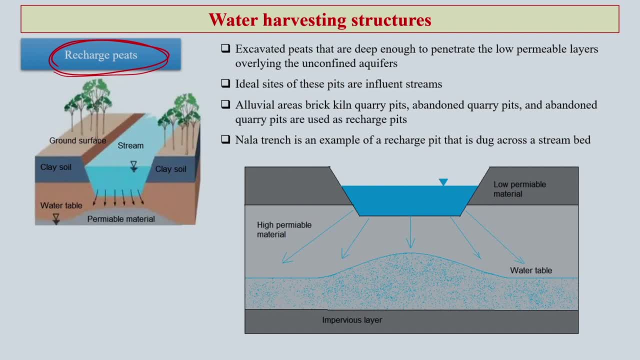 even the concave toy water from this aquarium is added to the reservoir here. So the滿, even if you have a low permeable layer, this recharge pits will allow you to take that water even into aquifer, crossing this, you know, semi-permeable or less permeable layers. 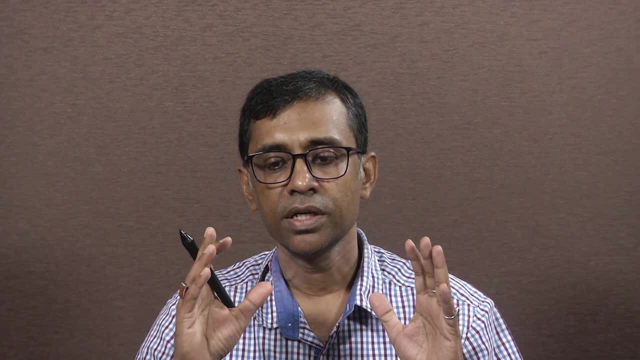 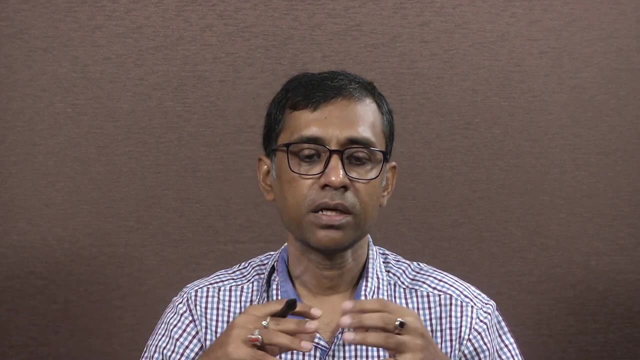 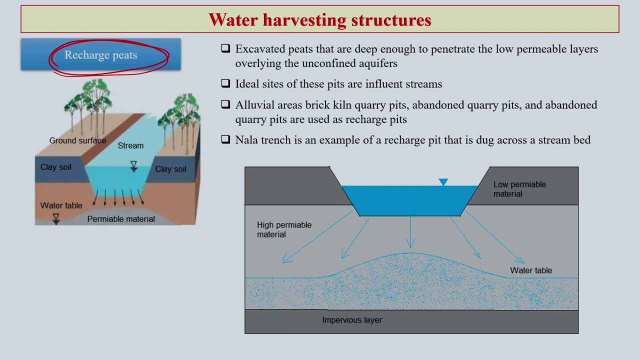 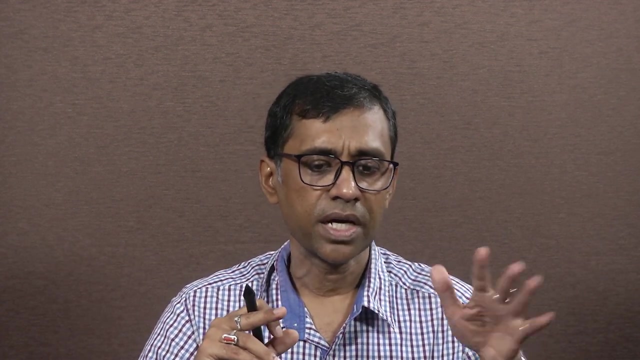 And these recharge pits are ideal sites which actually you know, influence those streams which you are actually having in and around that particular area- Alluvial soils or alluvial areas having lot of these days. you will find brick cleans, abandoned quarry pits and various kind of things, mostly in the alluvial areas. 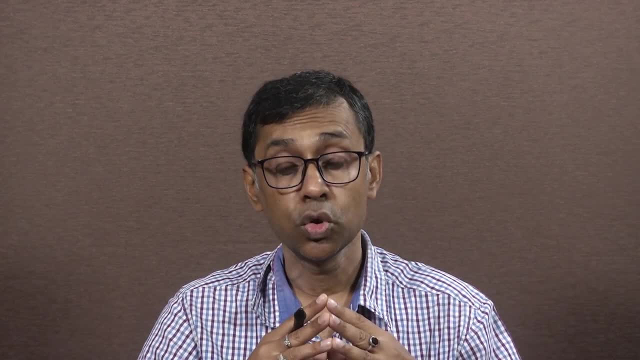 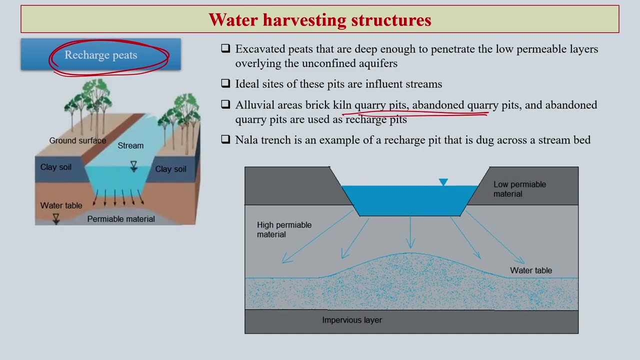 The reason is that the soil is very, very good for having this kind of small industry, But we all know that these are the things which these days coming in fact in between agricultural land. So that creates lot of problem with not only with polluting the soil but also the surrounding water bodies. 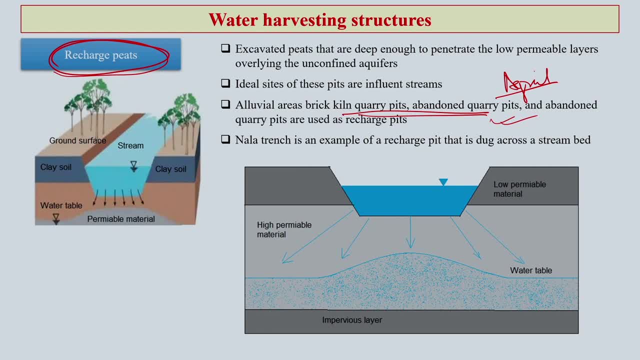 Now how actually we have created this kind of recharge pits. Now you see that this is the stream. you have any stream inside an area and then these are the ground surface. you have plants, clay soil, suppose, in the both side. then water goes down below the water table. 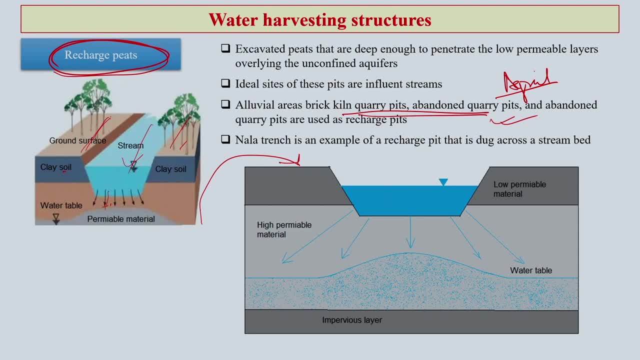 Now come here this picture, So you can see that this is the water table, which will actually clearly explain how this thing is happening in case of recharge pits. Now we have, suppose, high permeable material here, because I said that this is important. 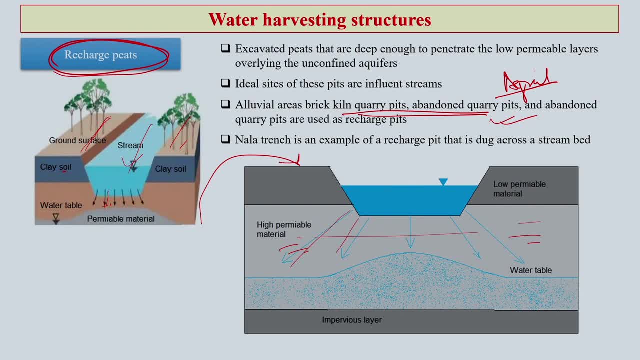 for groundwater to be recharged. So water comes through and straight away goes to the water table. And then you have impervious layer and these water tables- slowly it goes up and, utilizing these, recharge water table. You can have impervious layer and these water tables- slowly it goes up and utilizing these. 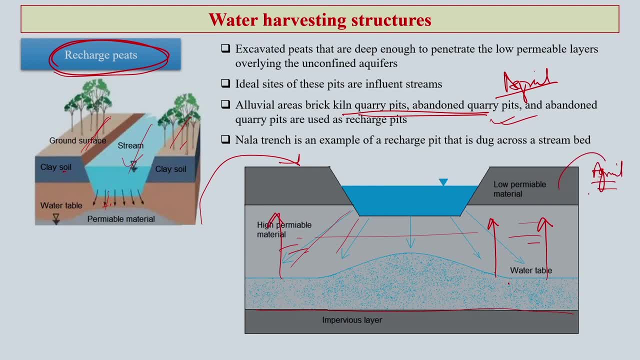 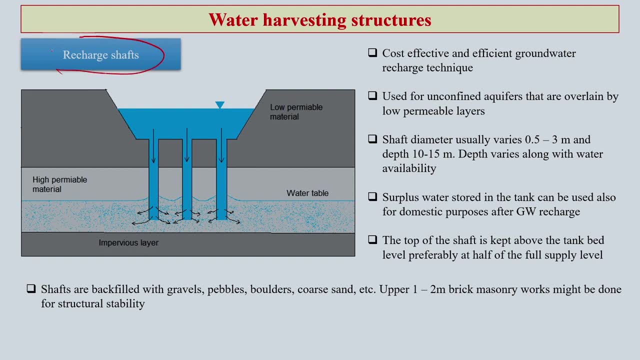 recharge water table. You can have your cropping system, agriculture or other activity utilizing this water. So next comes recharge shafts. Now, recharge shafts, as you see in this picture, is little different than the previous two. Here again we have the water body or the stream. here 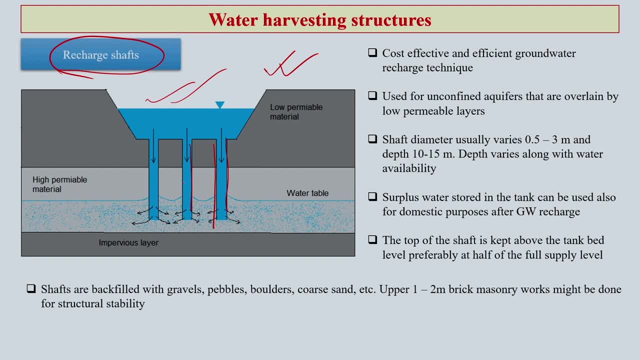 Here you allow through some channels the water to go into the water table directly, and here you can have in between also the high permeable material here and low permeable material here. So to bypass this low permeable material you use this kind of you know channel to 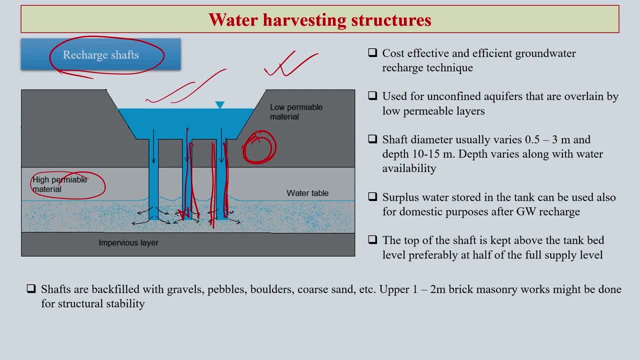 allow the water straight away go into the water table. It actually is cost effective and also efficient for groundwater recharge purposes. Normally, these recharge shafts are used for unconfined aquifers that are overflowing, And then you have the water. Here, you have the water surface. 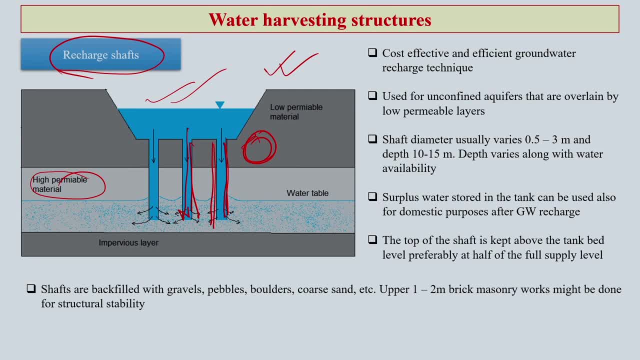 Here you have the water surface And then you have the water surface. Here you have the water surface And then you have the water surface, And then you have the water surface overlaid by low permeable layers, As you see here, shaft diameter. this is the shaft diameter. 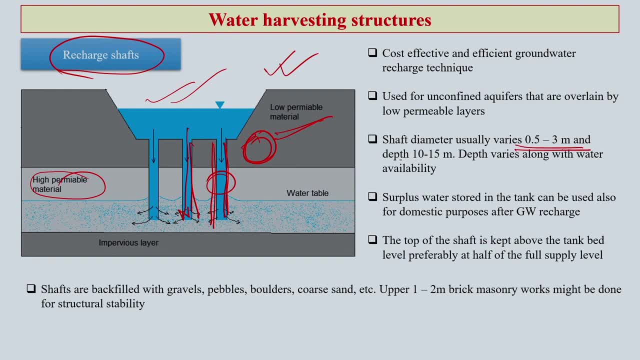 varies between 0.5 to 3 meter and depth 10 to 15 meter, So depth can vary along with the water availability. So your amount of water available there on the stream will decide the depth of your shaft. Now the surplus water which is stored in the tank can be used. 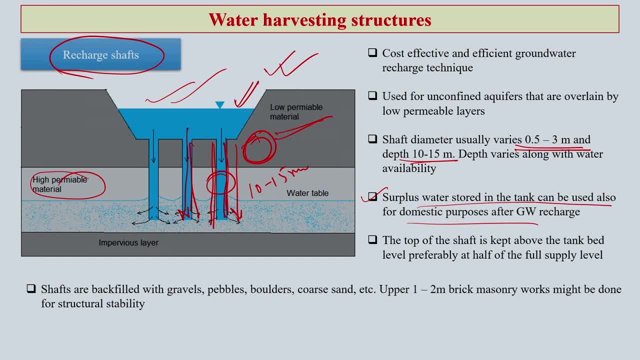 also for various domestic purposes and ground water recharge. as you see here in this picture, The top of the shaft is kept above the tank bed level, preferably, say, around half of the full supply level. So that is where you will keep your, you know, top of the shaft. So shafts. 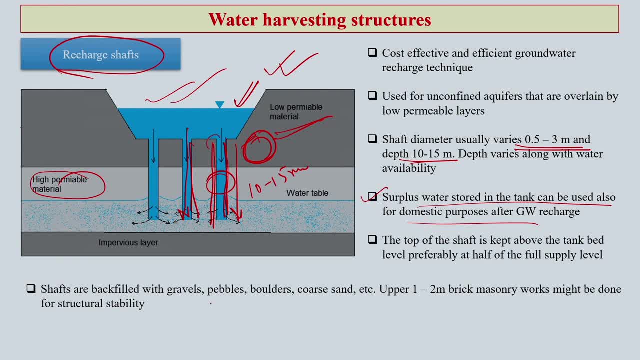 are again back filled With gravels, pebbles, boulders, coarse sands, and the top 1 to 2 meter is normally brick. machinery works might be done for stability of the shaft, just to give little bit more stability. So this is the way the rich shafts are being constructed and utilized for water. 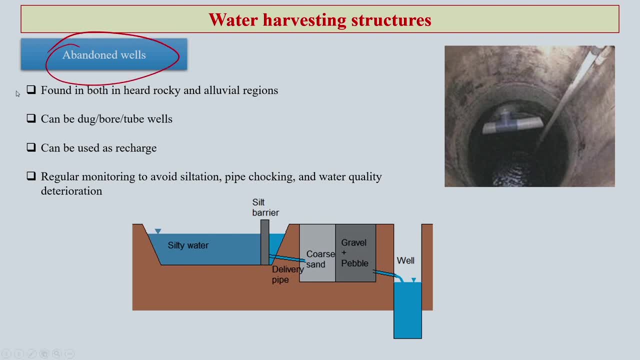 harvesting purposes. Next comes abundant wells. Now these are are very common in our indian villages and rural areas. you will find this kind of abundance wells many places across our rural areas and villages, found in both in case of hard rocky area and also alluvial regions. this can be dug or bored, as two wells we have also in the villages. 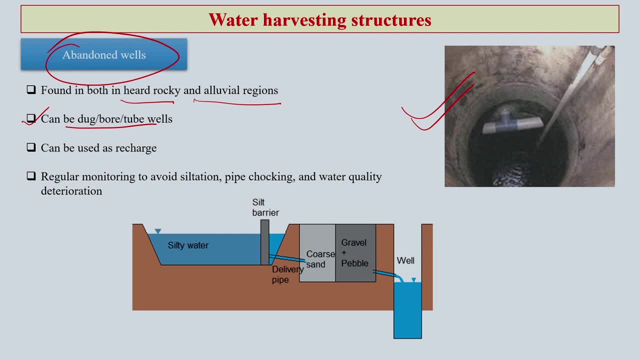 so same kind of thing that can be used, as you know, wells for water recharging. this can also be used as ground water recharge, which you have here in this picture. but one important aspect is that with this abundant wells, the regular monitoring is required, otherwise what will happen? that 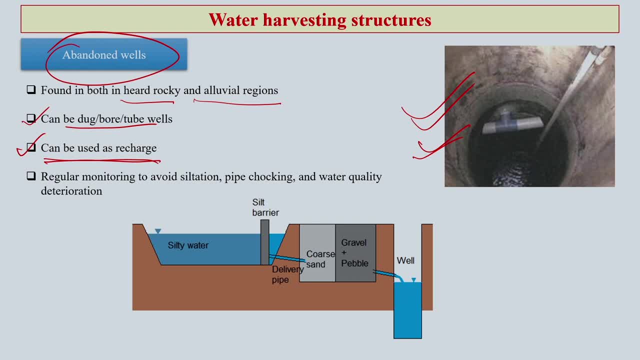 these abundant wells can have siltation. it also can have choking of the pipes. most importantly, the water can be reheating or pouring water, but the more it. Members should reuse the water once and for all if there is a big difference in the size of the water workload. 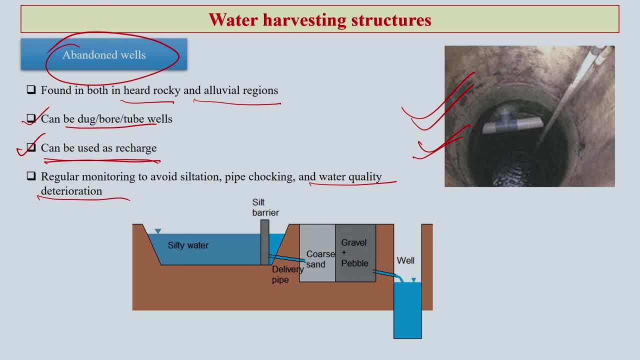 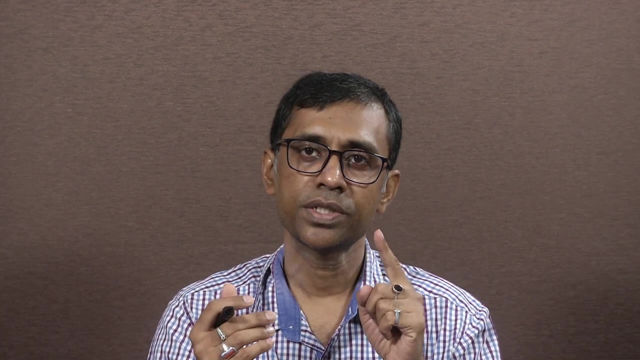 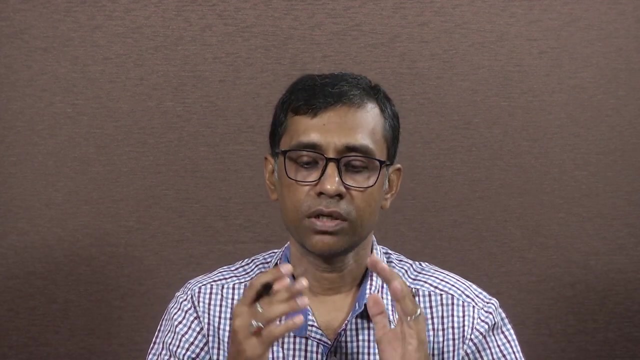 the water quality may get deteriorate. pollutions can also impact this water because, as I said, that if your water, whatever you have harvested after lot of effort and energy and resources, if you find those waters are polluted in nature, the entire effort of yours goes actually totally. 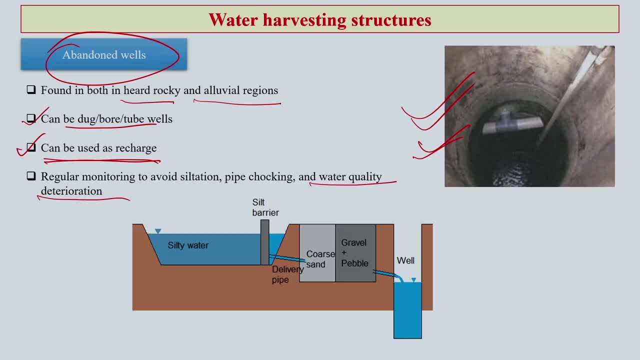 what you call waste for that purpose. So regular monitoring is a very, very important for this purpose. all right, so we can have, you know, various kind of situation for this kind of abundant well and this abundant well sometime, what happens is that if you have 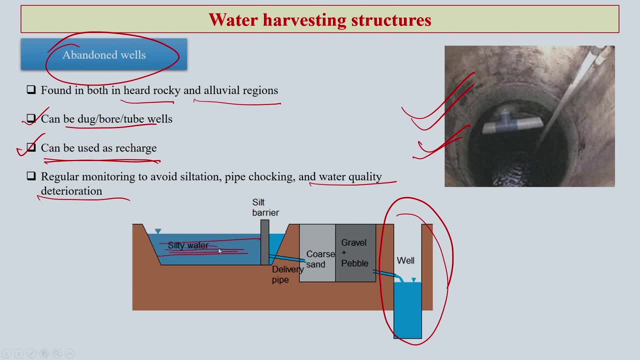 the stream and the water nearby, the source of water nearby, then you can have some delivery pipes from the ust음�, memorable music for this passagepeople looking at it from this. another question: can you tell about how Civetav denominator can be mustard or any source of water which can be relieved from the source? 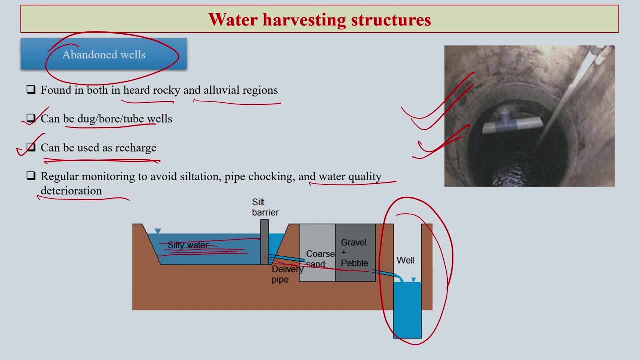 water stream and it can pass through core stand and gravel and pebble and then finally can go into the well. So this is the way a kind of small filtering of the water that has been harvested can takes place and you can avoid the chances of contamination of. 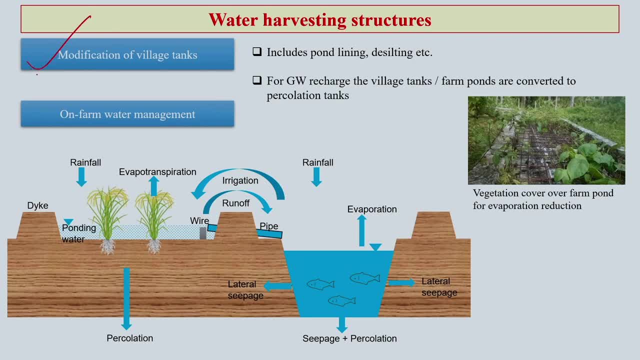 harvested water, Modification of village tanks and on-farm water management: These are again very common in our Indian condition. These modifications of village tanks, on-farm water management, normally carried out through lining of pond, desilting of pond, then tank and farm ponds. 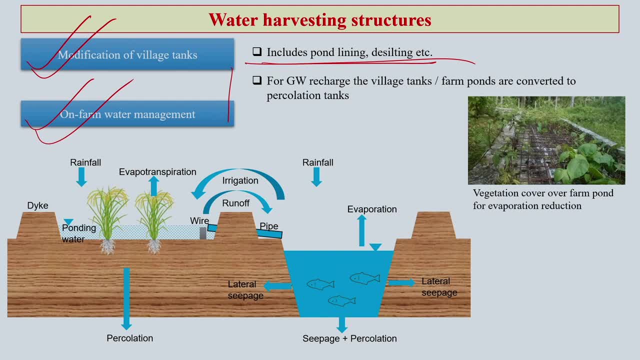 which percolation ponds which are actually used for ground water recharges. So what happens is that this picture will explain you in detail about this type of water harvesting structures. Suppose, in an area you have a, a pond area where you have water, rain water also gets stored. You can actually grow certain 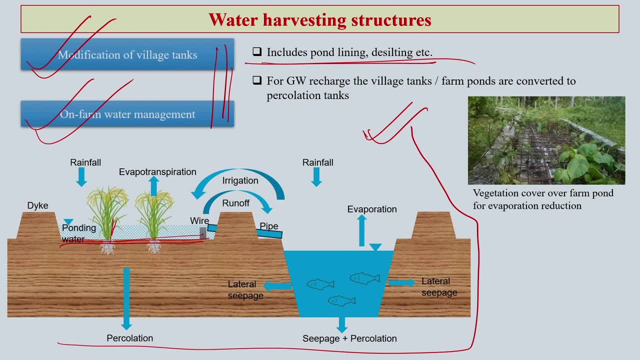 kind of plant species which love flooding condition, like the rice. So, apart from growing the crops in that flooded area so that water which is stored in the pond area, you can protect them through some dike system. Also, you can have, you know, some 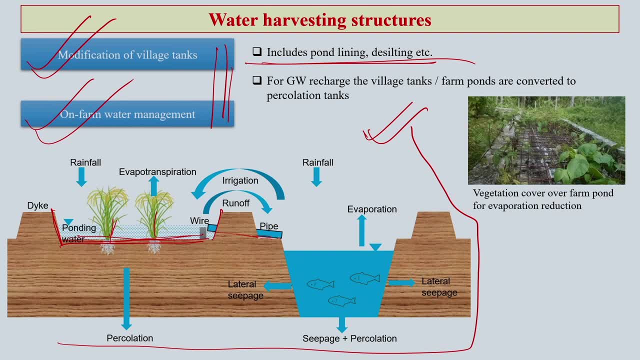 piping system from this water body, take the water into a seepage or percolation pond. Now, once this water comes here, you can actually use it for aquatic lives, fish and etcetera, some other uses. So this percolation, once it comes into percolation pond, then you know. 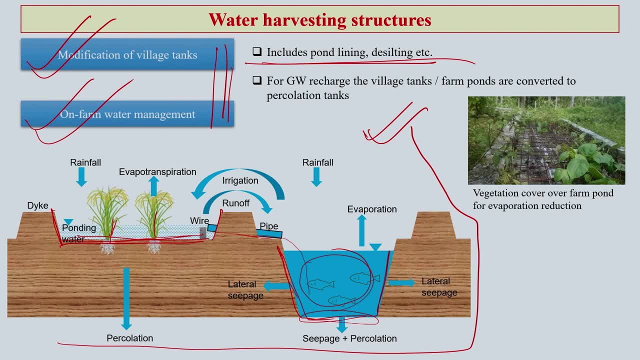 that it is going to recharge your groundwater both way. it can go vertically down and also horizontally on both side. So what happens is that this on farm management of water harvesting is very, very sustainable in nature and it could be very useful for overall development of the water resources in any rural area. The reason is that in one hand you are able. 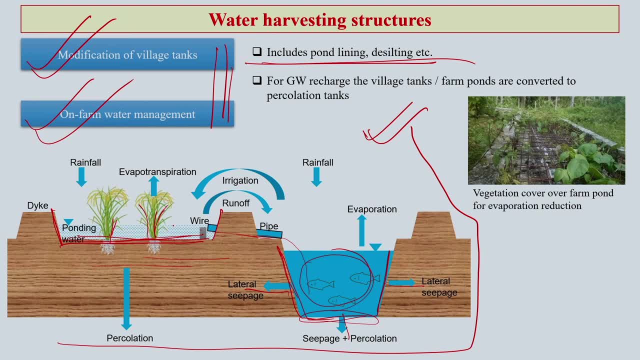 to get a crop which can withstand flood water or flooded condition. On the other side you are also having your groundwater recharge. So this kind of situation can be created very easily in any Indian rural area or villages And sometime you will find that you know some of the small ponds or tanks are often having 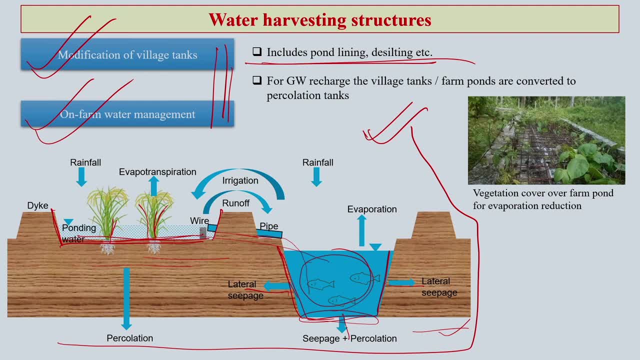 kind of vegetation cover or aquatic life. So you can have actually livelihood also from utilizing that the water, the rain water which is stored in the pond or in the percolation pond. so overall this can be a kind of a win-win situation. in one hand you store, you harvest the rain water. 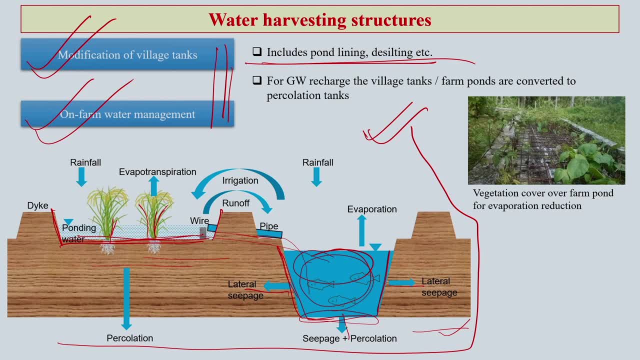 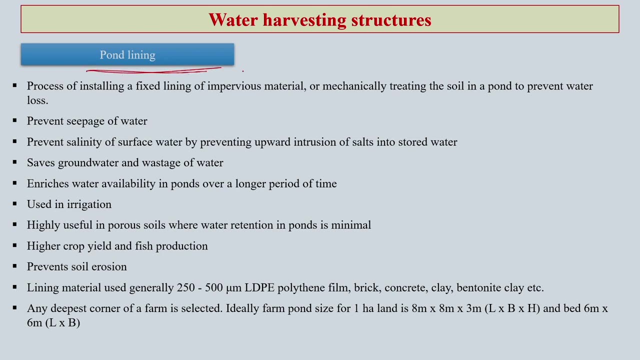 on the other hand, you generate income utilizing the water that is stored, apart from recharging your ground water for you know, future agricultural practices- irrigation. so this is how you see that different water harvesting structures. it actually helps. pond lining is also important in case of water harvesting structures in rural area, so the lining of pond is critical to avoid. 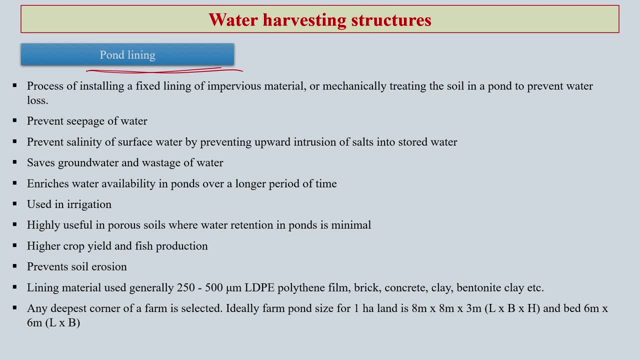 you know the the erosion of the soil and also you allow the water toe gets stored in that particular pond for a longer time. now it stops or reduce the seepage of water. the pond lining it also puts water in the soil so it does not affect the water that is being harvested. so this is one thing. 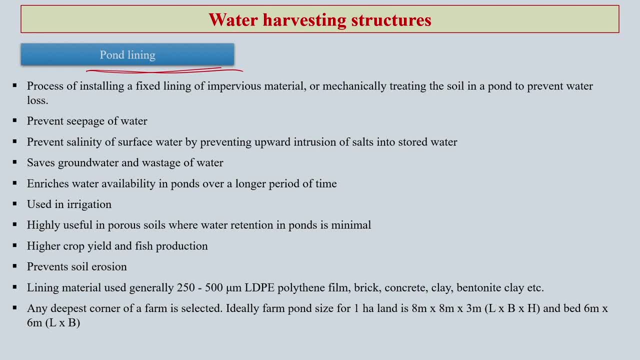 prevent salinity of the surface water by preventing, you know, some upward intrusion of soils in the stored water that you have created in the area. It also saves groundwater and wastage of water. Excessive water evapotranspiration can also be regulated to some extent. 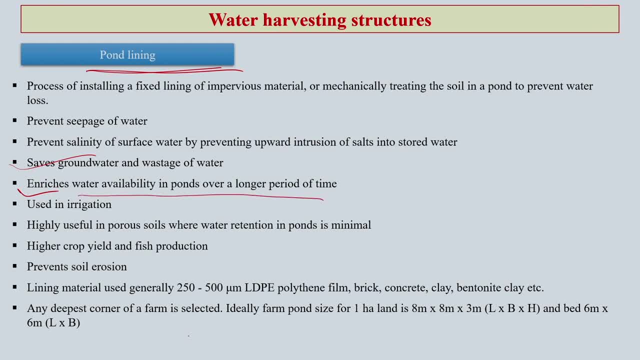 It enriches the water availability into ponds for a longer period of time. Similarly, this water can be used for irrigation more efficiently if your ponds are, you know, having linings, Highly useful in case of porous soil, where water retention in ponds become a challenge. 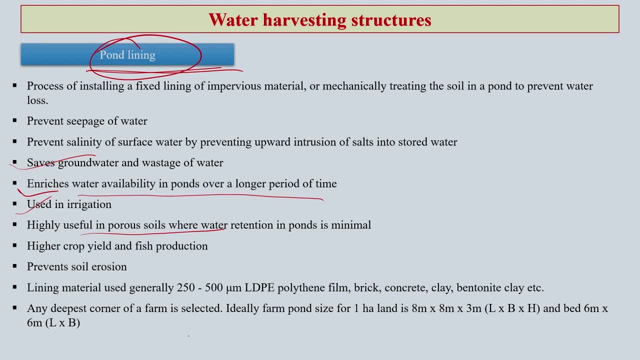 So if you have pond lining, then you can actually allow the water to stay there in the pond. Otherwise it will pass very quickly from the storage tank. It prevents, as I said, soil erosion. Lining material: we use different kind of lining. 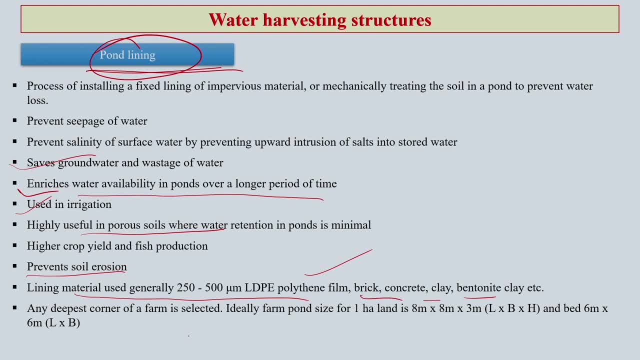 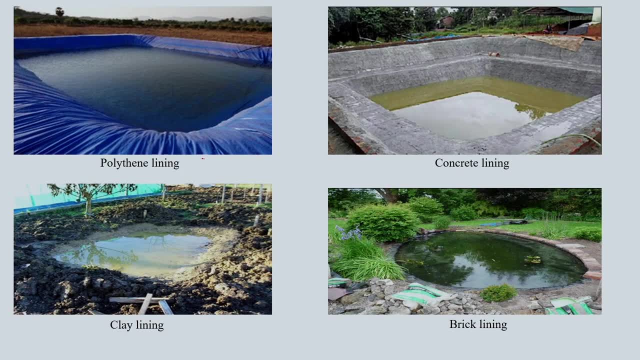 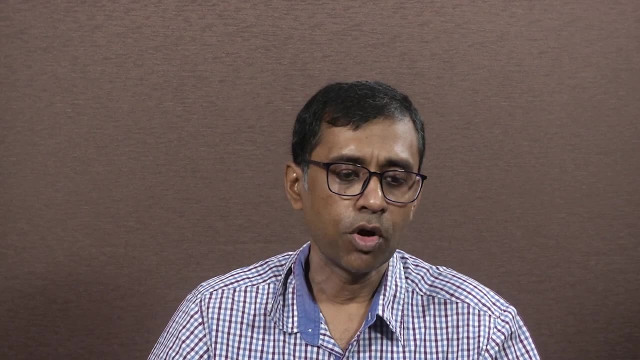 material: Polyethylene, flim brick, concrete clay, bentonite clay, etc. I will show in the next slides couple of examples of those Polyethylene lining this is. you know this looks like this, But if you ask me, I would not go for polyethylene lining as the very first preference. 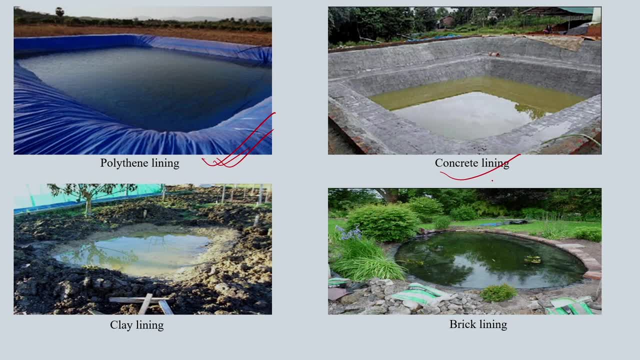 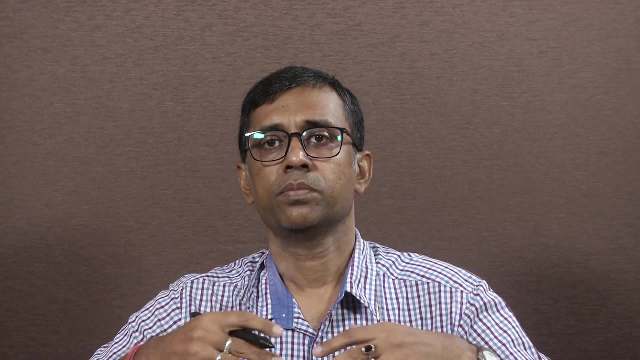 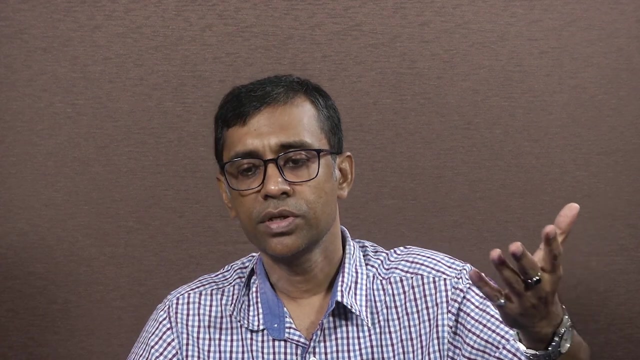 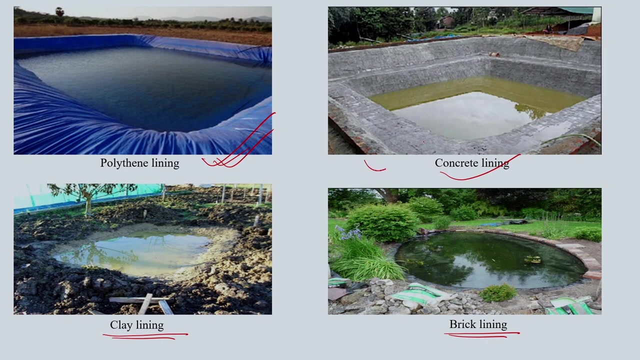 Neither. I would go for concrete lining again as the first preference. So what I will prefer at the village level is that clay lining, But No the, Because of course they are actually allowed the water to stay there And I think that I eh think the solution is for a WE land. for that reason, 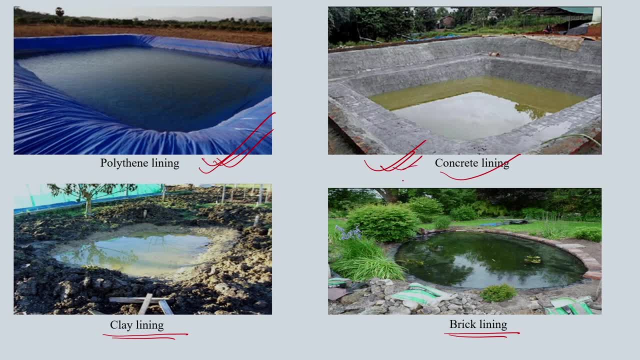 But if you need your larger amount of water storage, Then you need, in a larger area of agricultural practices than you need, concrete and polythene type of lining, because of course they are actually allow the water there to stay injured. So unless you are asked and the applicant is the one who has one duty, 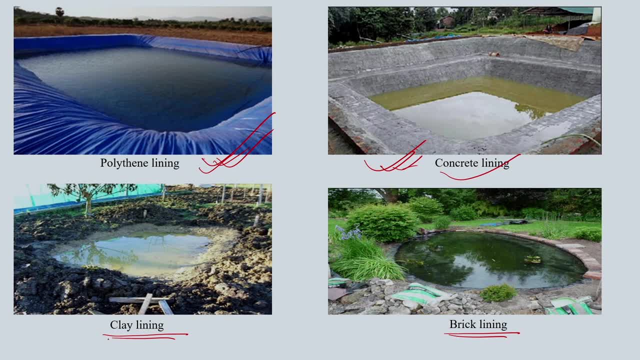 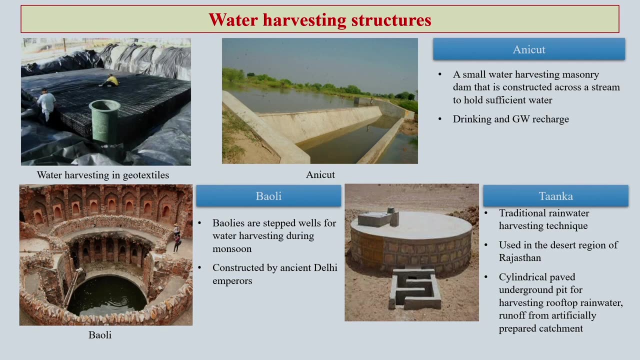 So the strikes, Yes, to get stored for much longer time, but clay lining and brick lining- these two are the cheaper option and also sustainable in many ways. these days there are many kind of new materials are coming, also using for water harvesting structures, geotextile, geosynthetics. these are some of the 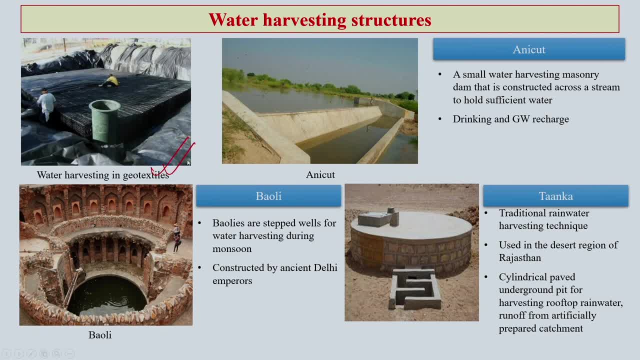 things which are coming, you know, increasingly in case of water harvesting structures, anicate. we are already using in many cases in southern part and and also in the western part you will see lot of uh indicates. these are basically small water harvesting masonry dam which are normally constructed across a stream and the water is largely used for irrigation. 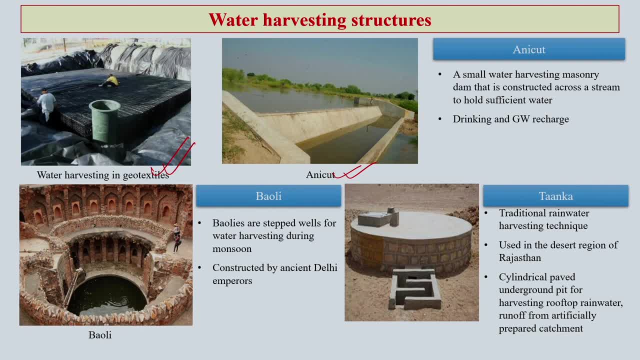 and also for drinking purposes in rajasthan, especially if you, if you have been there, you will see that you know hundreds of years back, the ruler of Rajasthans, the kings. they actually used to have a kind of water storage structures which they call. 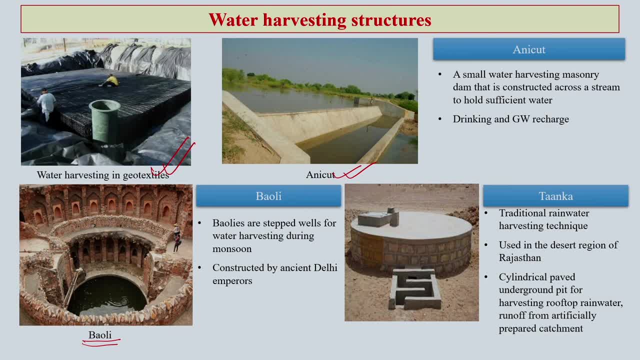 Bauli. Now this is amazing to see that even hundreds of years back they had such kind of technology knowledge with them. These Baulis actually could store water almost the entire dry season, So they could actually utilize this water for many, many months when the outside. 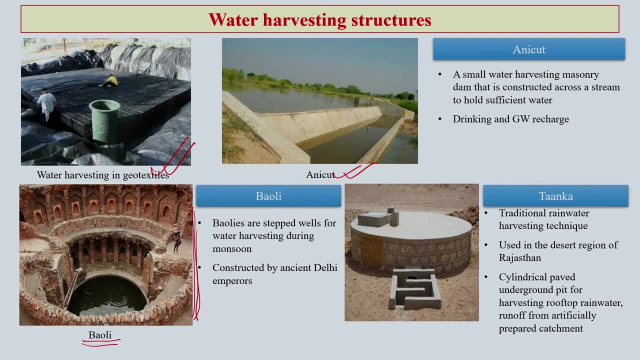 weather is very harsh, completely dry. But Baulis will have water there which is stored from the you know very little that window of rain that they used to get. Baulis are kind of you know stepped wells for water harvesting So they make it stepwise as you see in this picture. 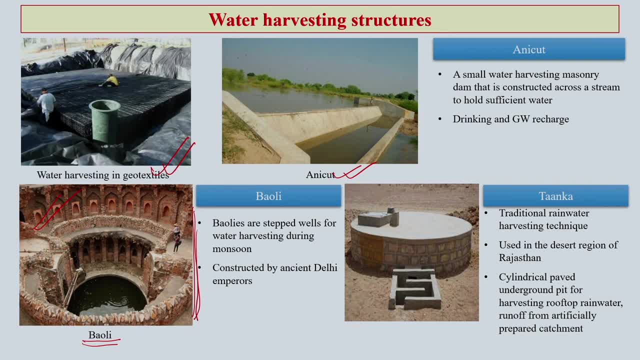 So some of the water harvesting structures in the northern part of India. often, you will see, they call it Tanka, So these are the structures that are used for water harvesting. These are traditional, again, rainwater harvesting techniques largely used in Rajasthan and sometime in UP areas. 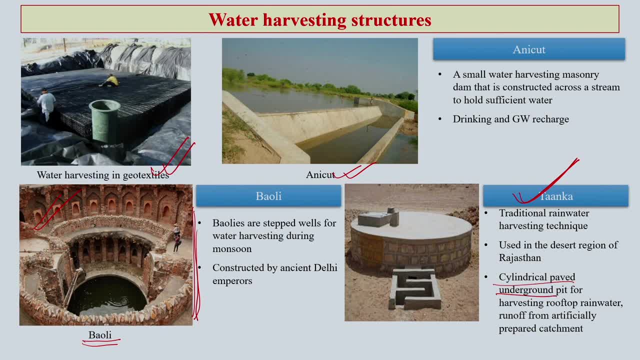 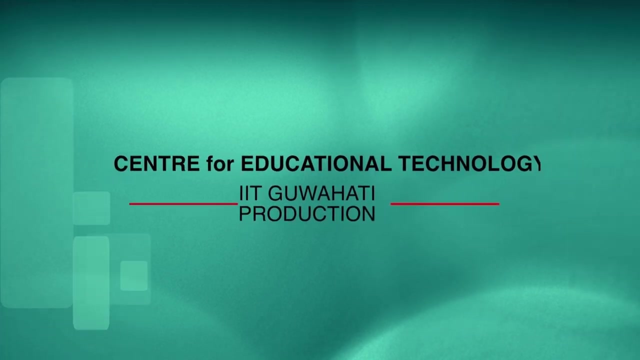 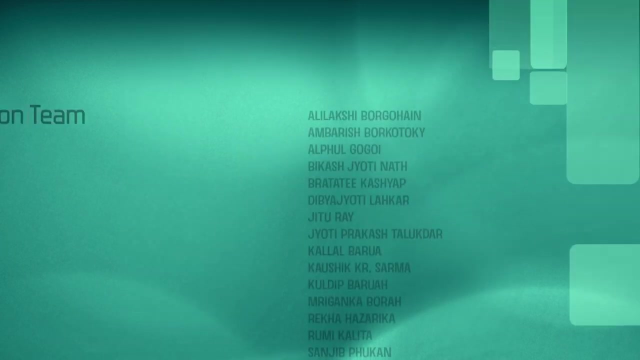 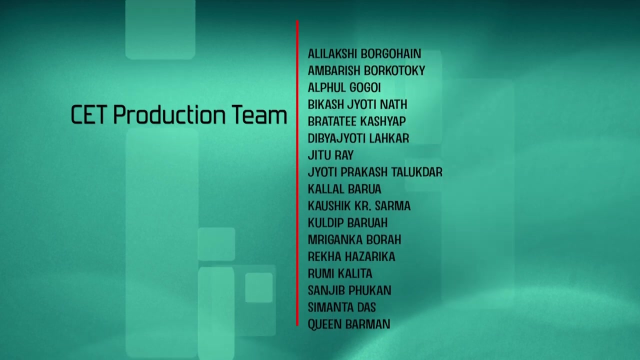 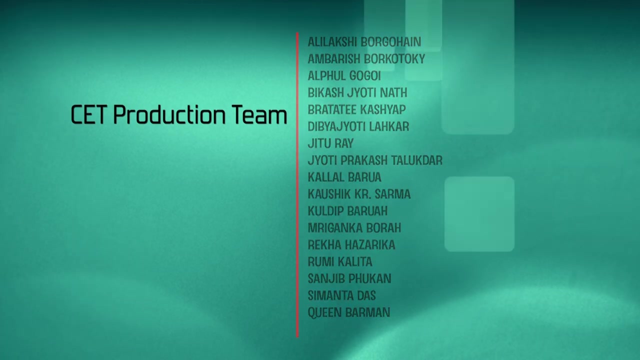 This is basically cylindrical paved underground pit for harvesting roof water, rain water or runoff water which comes in and then they can pass through this and then they go inside and stored in the tank. So this kind of structure we call as tanka. Subtitles by the Amaraorg community.